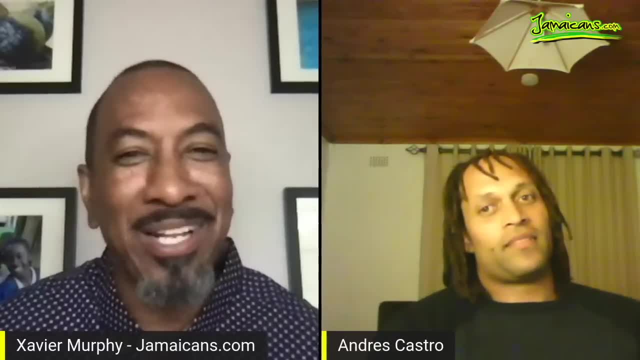 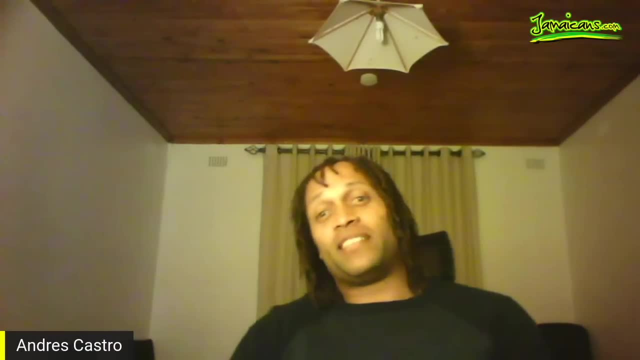 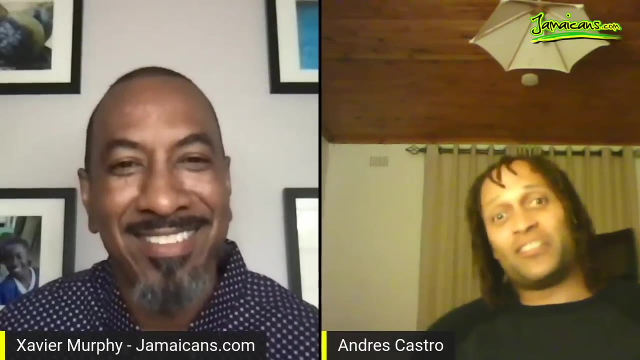 All right, And are you representing any high school in the Kingston area? Well, the difference is I moved to Mandibu, Manchester, so I went to West Indies College High School and did a stint at Knox College as well- At Knox, Yes. 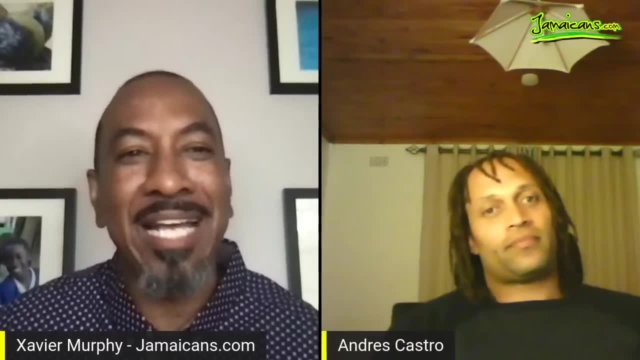 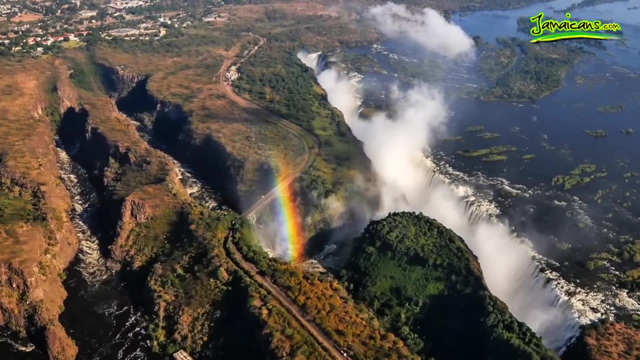 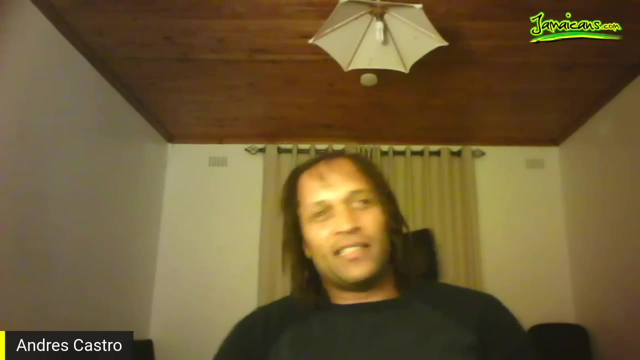 All right, So tell us your story. How did you get to Zimbabwe? So it's through a job, through a mutual friend of mine. I was offered the job probably about three years ago. I didn't really take it until Until a friend of mine who is an African- I call him my Kenyan brother- decided to say: 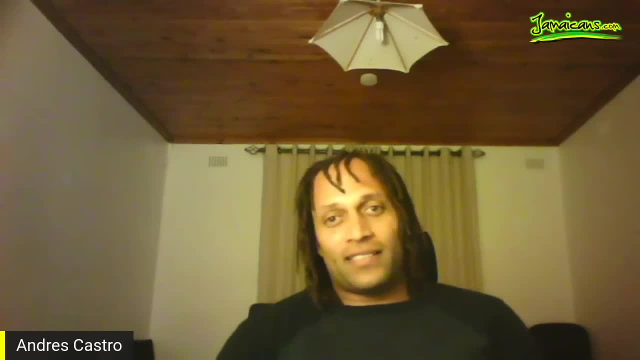 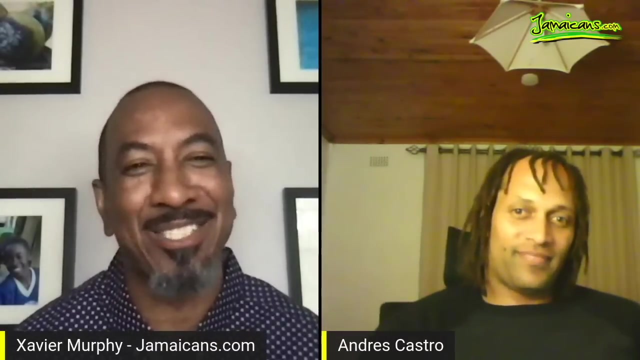 you know it's time you go back to the motherland, And, being that Jamaica and Zimbabwe had loads of history, it was time for me to venture Nice, Nice. So you dropped right into the loads of history. Talk to me, talk to us, Tell us a little bit about what you have learned. 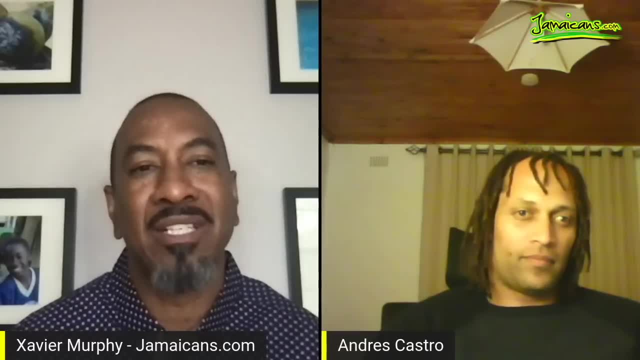 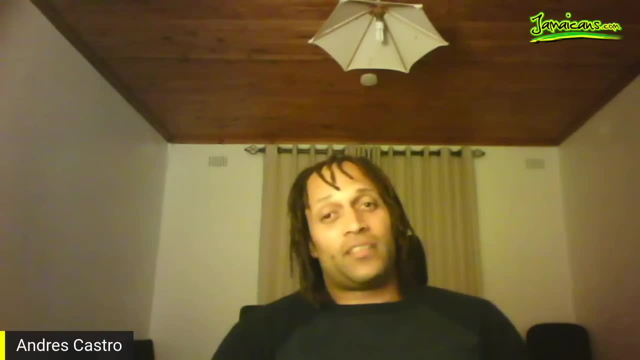 You know, living there, about the Jamaican history and how the Jamaican people are viewed there. I would say Jamaicans are highly respected and very, very highly viewed here in Zimbabwe As soon as people find out you're Jamaican. you know people here speak. 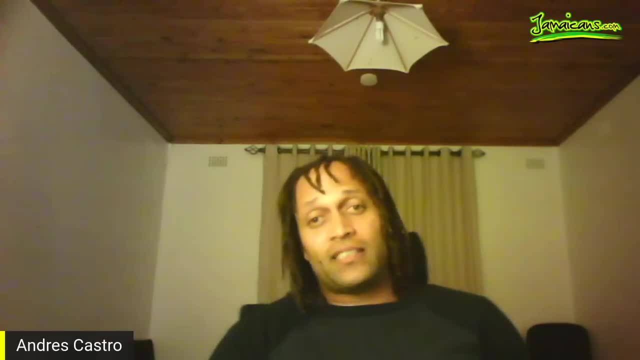 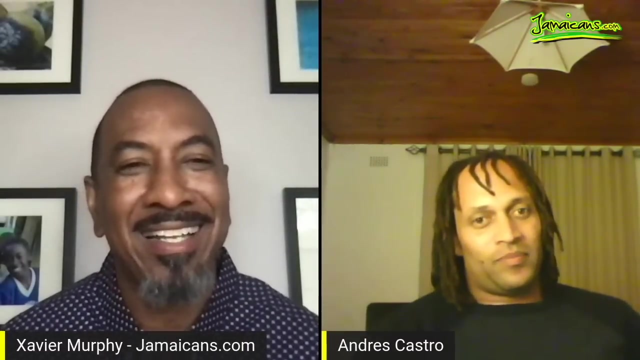 Patwa Also. they're very into dancehall Big. They know All of the latest songs, all of the latest artists and so on. So the one story that always comes back to me when I hear the country Zimbabwe I have a friend from, 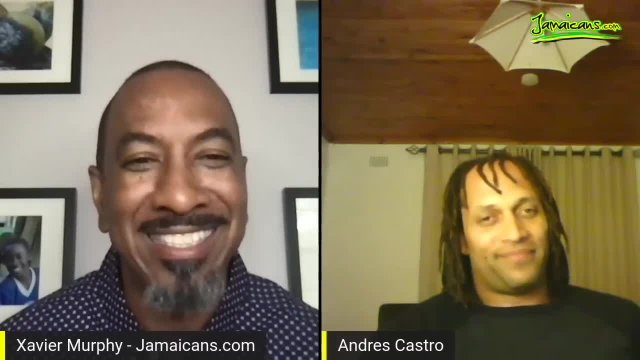 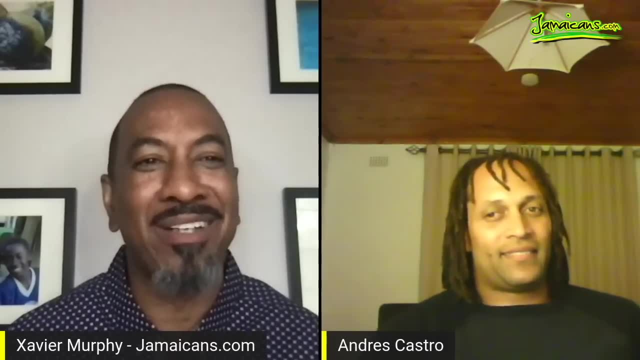 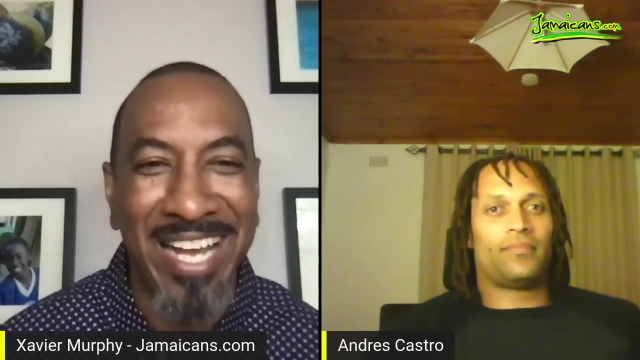 there also is Bob Marley, The performances that he did there when the country gained independence, And, and, and also the story of on the way where prince charles wanted to to to meet him, and i don't know if you've heard all these stories and. 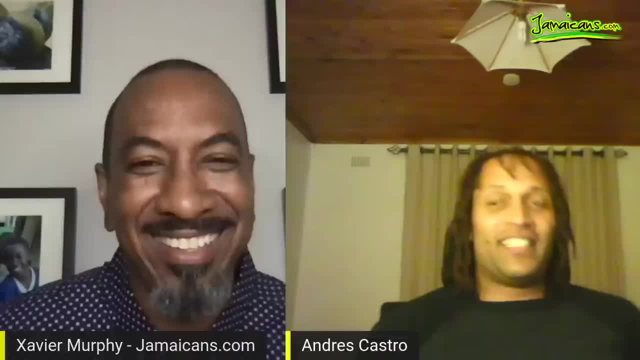 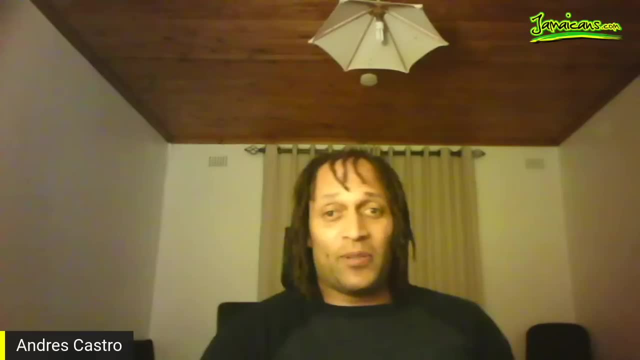 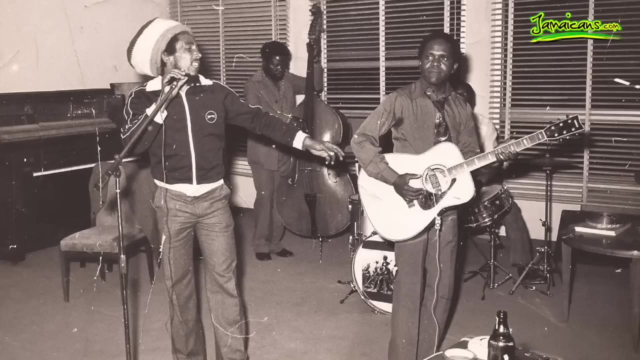 and well, well, there's, there's a good friend of mine i need to to sit with be because he was here within that time so i still have a few more catching up to do with him when i'm not busy to go through all those uh, musical histories with zimbabwe and bob. okay, okay. so on the people, 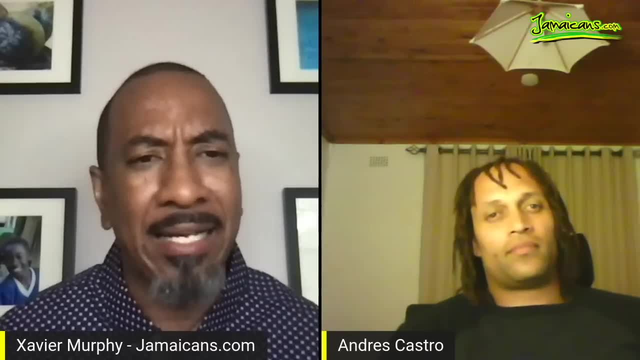 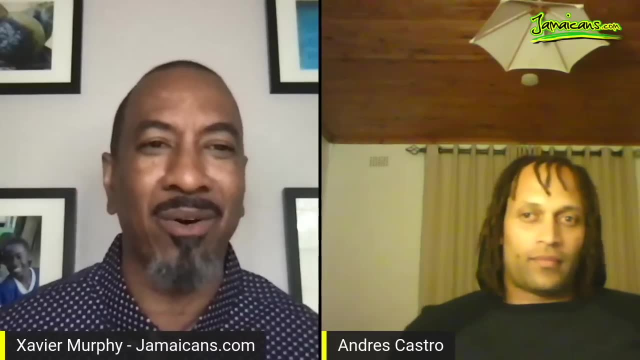 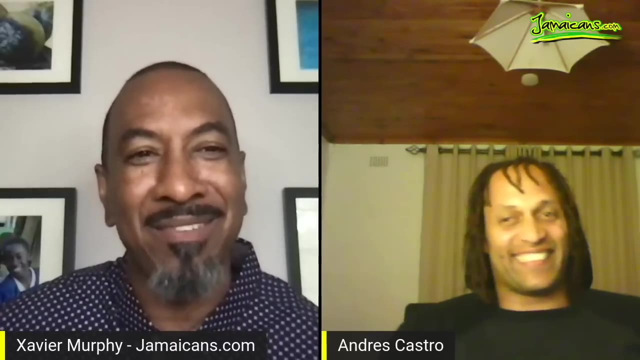 itself. you know what are the people like? you know, are they warm? you know, you know you have to get to know them for a little bit. are they up? you know we're a little different. as jamaican, sometimes i say we're, we're up front, we're gonna tell it like it is, and so on. so what are the people in zimbabwe? 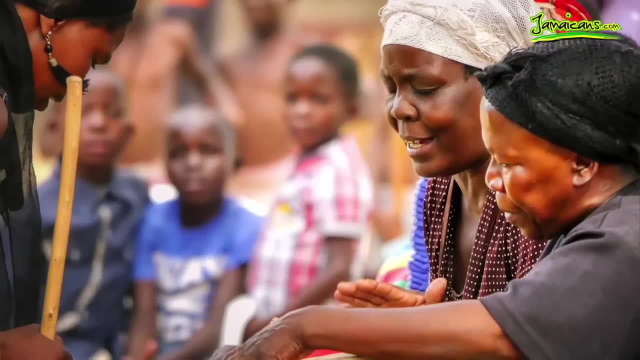 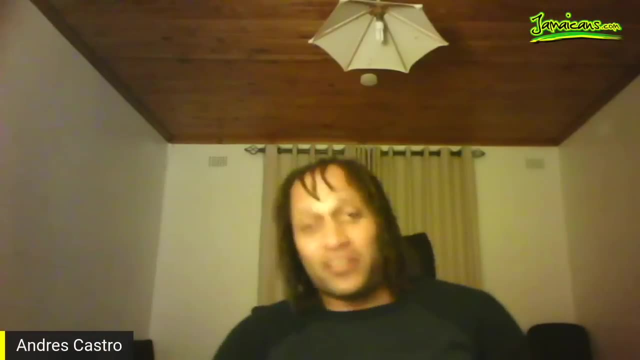 like um, very warm and very friendly, um, even to the point where they have what we would call their umpires umpires. i've been down to barry and i people have given me the, the big misconception. but, being a jamaican, as as i am, when i i went to barry the, the, as i say, the getter youths. 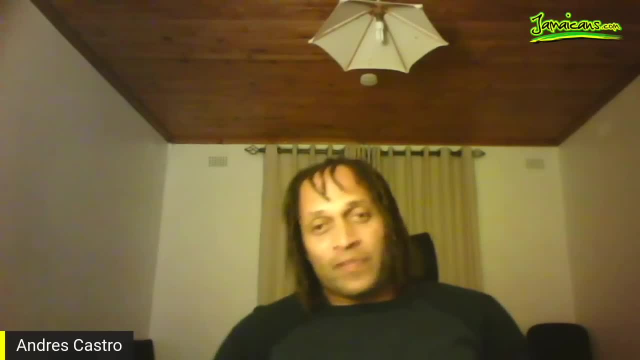 they came up and they found out i was jamaican and they were really warm and welcoming. they were even starting to sing vibes cartel, and my border sounds to me, and do i know this tune. or have you heard about damian molly, sean paul don youth, you know. 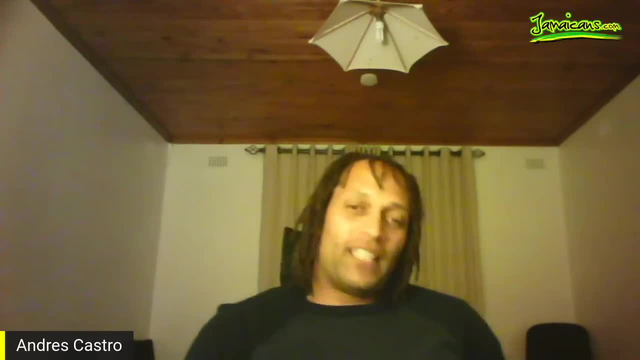 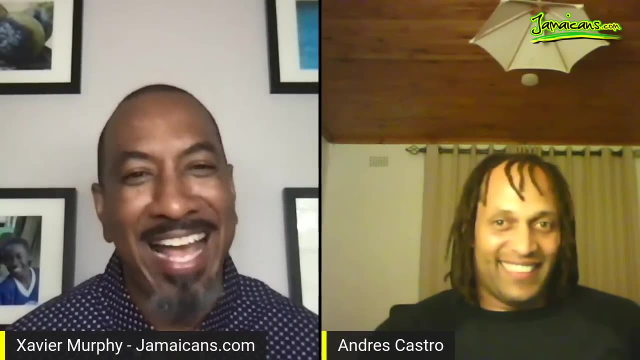 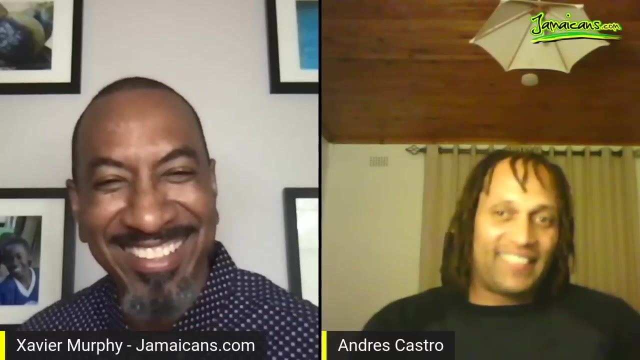 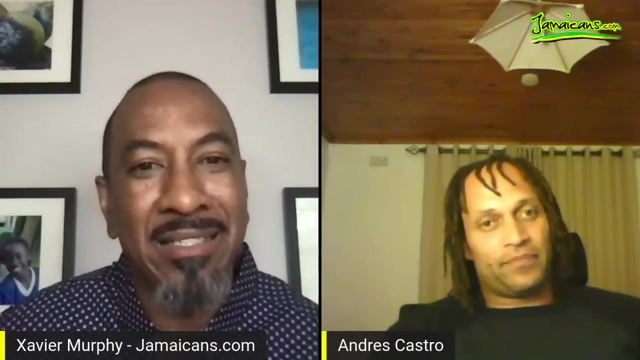 the musical scene was very fruitful. that's what they wanted to know, so it sounds like i could visit there and be driving and and hearing a popcorn, or yes, yes, puppy, puppy is big here. you know any of them, any of them came. any other jamaican reggae artists? 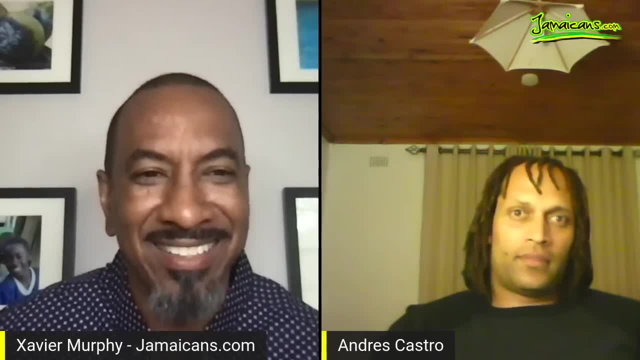 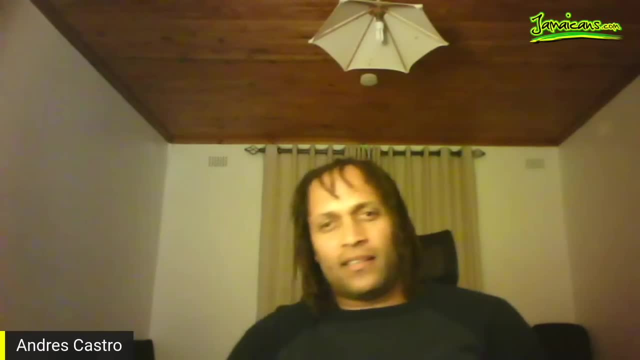 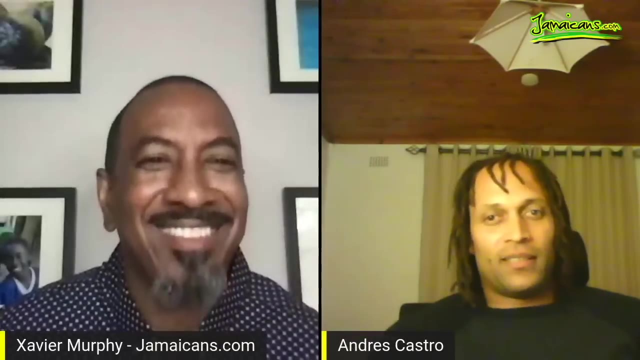 uh, visited recently. find the type of concerts? uh, no one recently um, but what i've heard is that sizzler capleton came um, which you would expect because you know sizzler and capleton have always been preaching about africa. so it's yes, more than likely you would expect to hear from them. yes, 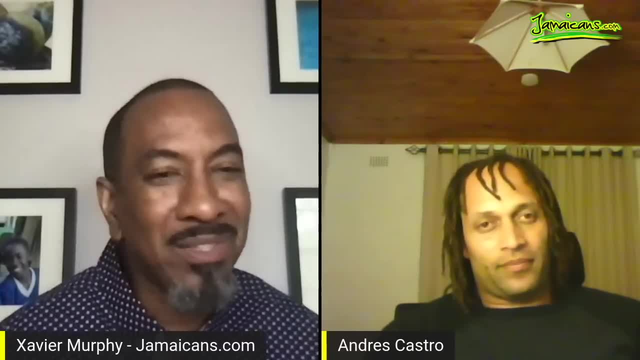 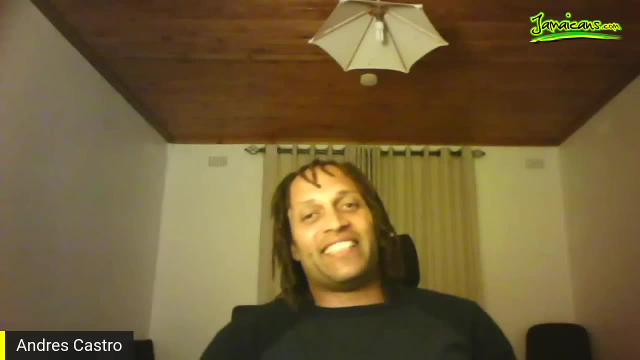 so i went jump to food. tell me a little bit about the food, and what's the food like there? well, um, it's, it's more to do with beef. so i'm i'm a vegetarian, so you know me. obviously you can see my locks is growing, but shout out to my mom who raised 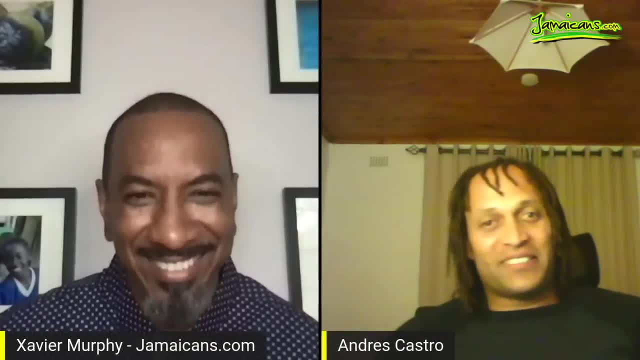 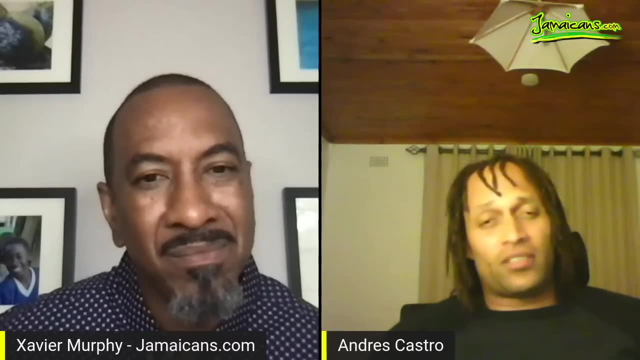 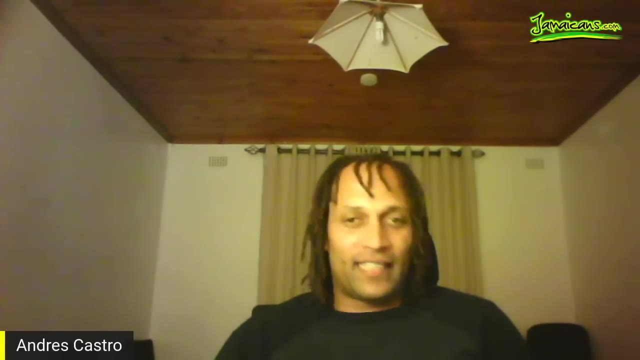 me as a vegetarian, so she'd be proud of that, you know, okay. so for me it's more like uh salad, so it's rape and stuff. but they also eat something called well. to us we would say it's like turn cornmeal, uh, but it's called saza, so it's it's like cornmeal turned up, you know, and they dip it in. 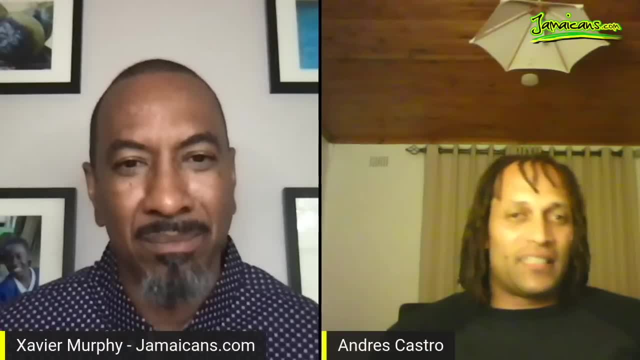 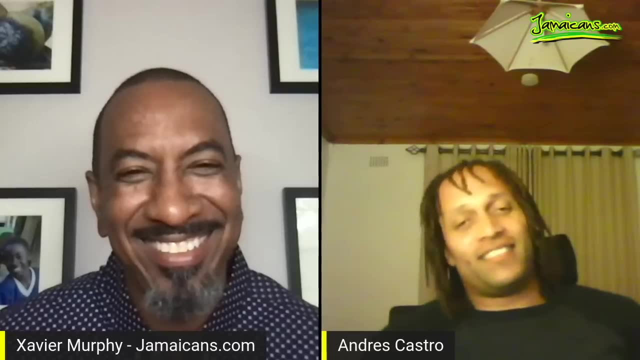 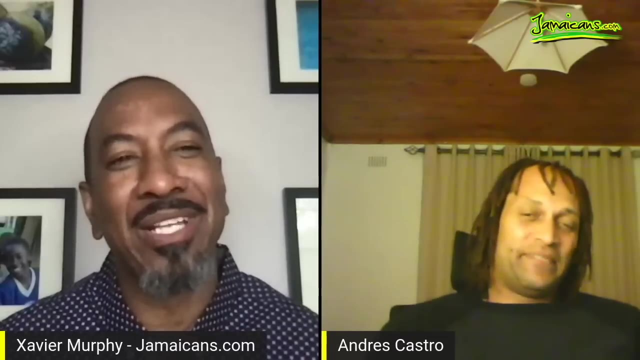 there's a they. they're very big into eating meat. here. it's a lot of beef and chicken, you know. so there's no better food than our jamaican cooking. i'm gonna be biased, yeah. so then let me ask you this: i know you're not a meat eater, and so for us, uh, carnivores as they. 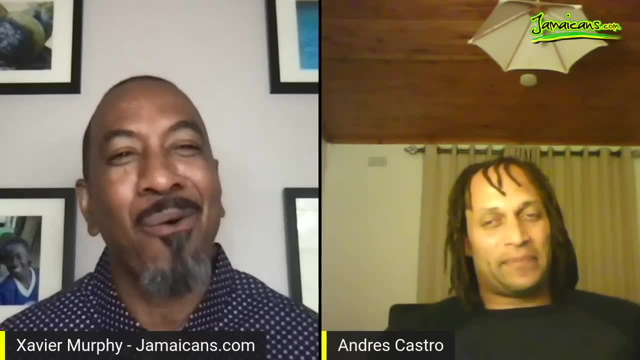 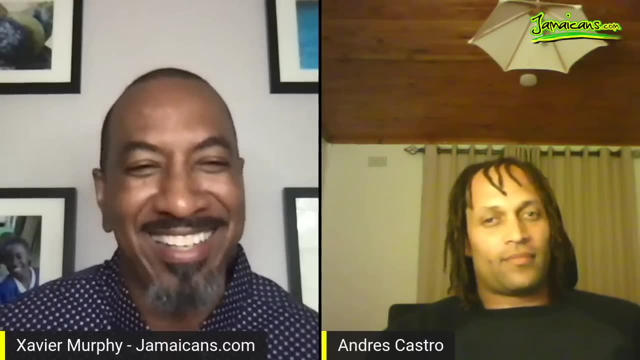 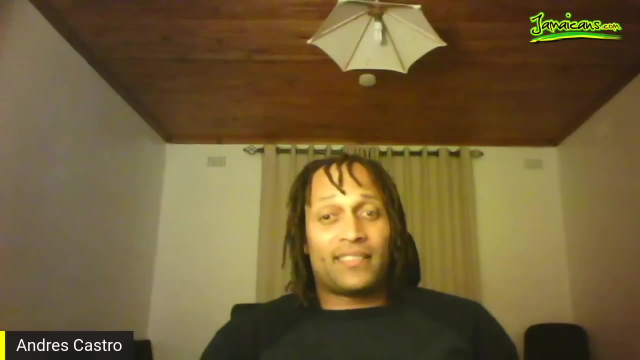 may call them our meat eaters like me. um, what do you hear people rave about? like? this is a dish that is just really good. the one thing that resonated with me is that they, similar to jamaica, they eat a lot of oxtail. um, uh, there's oxtail. 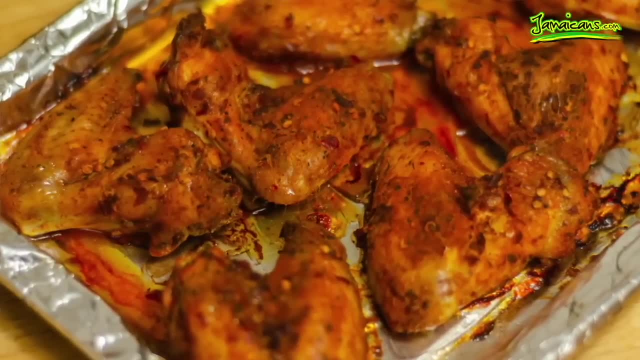 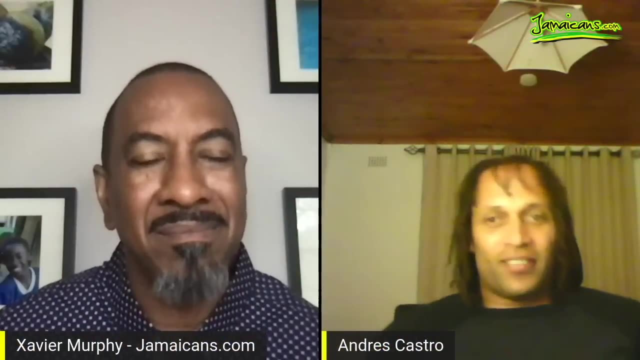 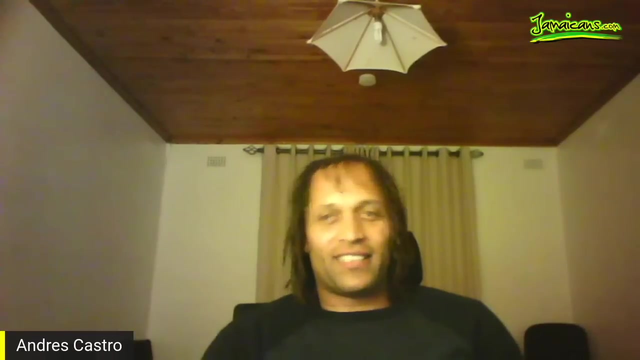 there is, uh, peri peri chicken because, as you notice, zimbabwe has that connection with mozambique, which was conquered by the portuguese. so you have that peri peri chicken, um, and i think it's it's starting to get a bit too commercialized, because you can see kfc um, no, mcdonald's obviously. 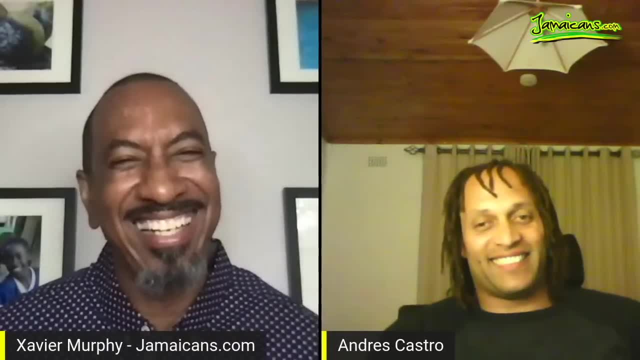 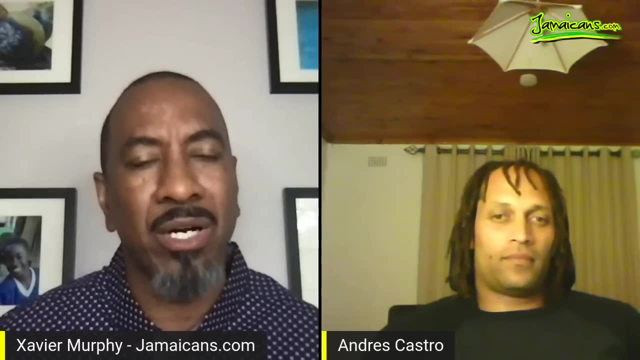 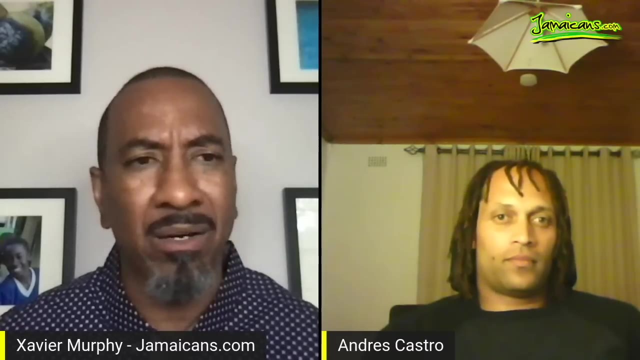 but um, okay, let me ask you this, because you kind of touched on a little bit that you know mozambique is next door, there's curry and so on. what's the population um like? is it like there's expats there? folks from other other countries are, are. 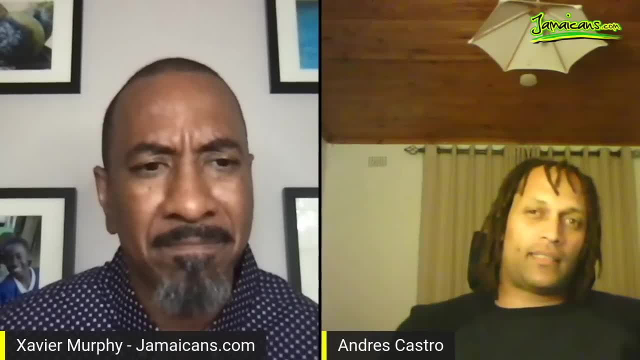 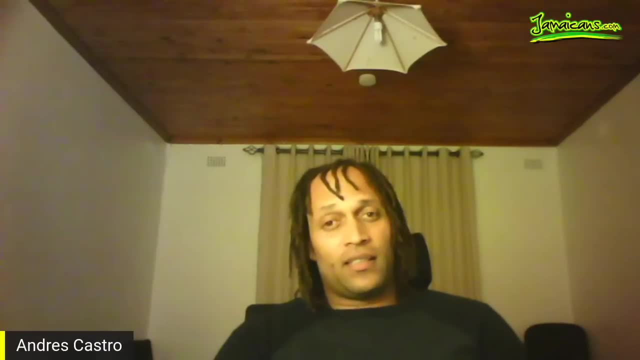 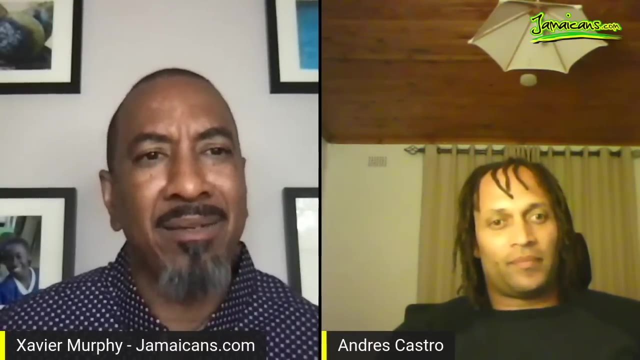 there also are it's, it's, it's a big diverse community. you can have anything from swedes to swiss, um americans, it there's. there's a big expat community, okay, and? and folks, i'm not saying all of zimbabwe, i'm just saying maybe we're 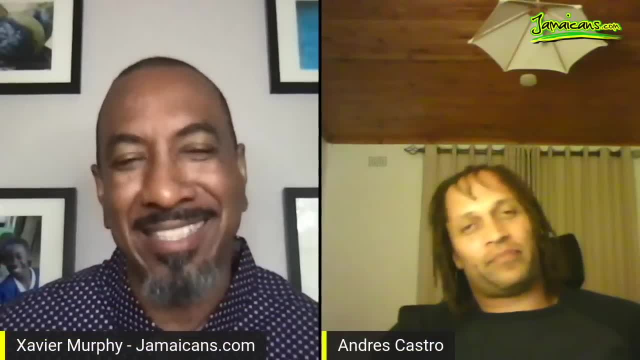 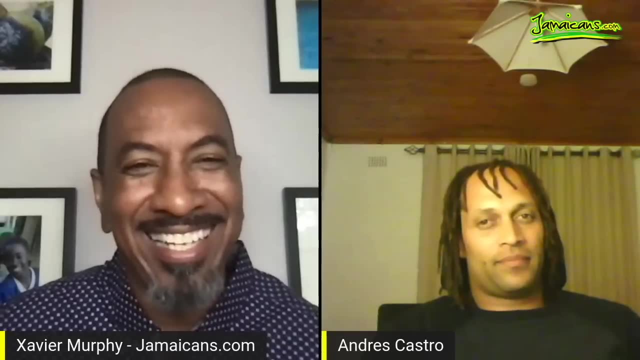 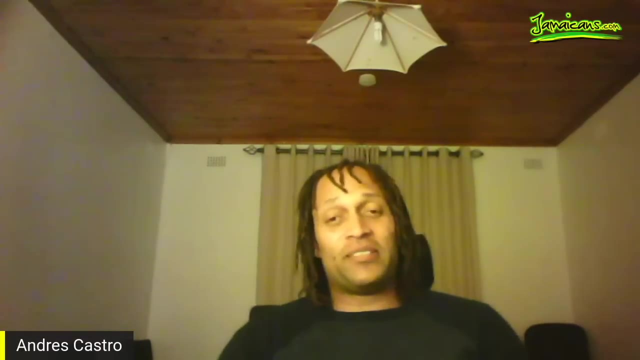 where andres is. that it may be, you know, in a city where there's diverse, you know, population and people um language, what's the language? so it's shona, but, uh, they're shona, but, knowing zimbabwe, there's different dialects that are spoken um. 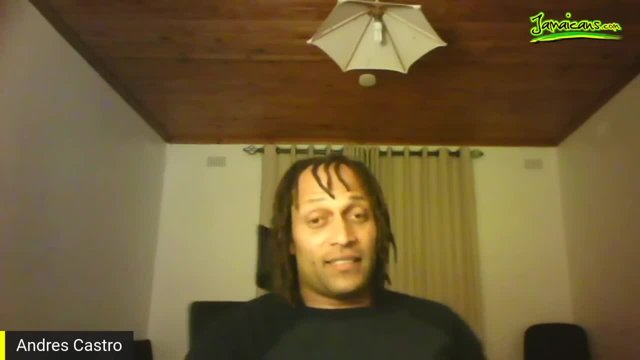 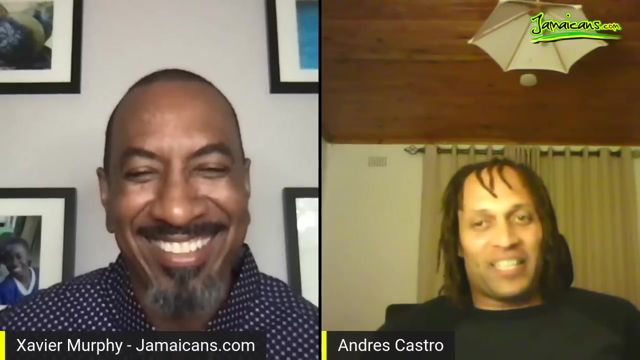 um, so, um. so that's the main. one is shona. the second biggest one is uh, the belly, which is uh similar to zulu language- um, which is good, but it's a lot of clicking sound with the zulu language, you know. so i'm still working on my show now at the minute, you know. okay, so you, you is there. 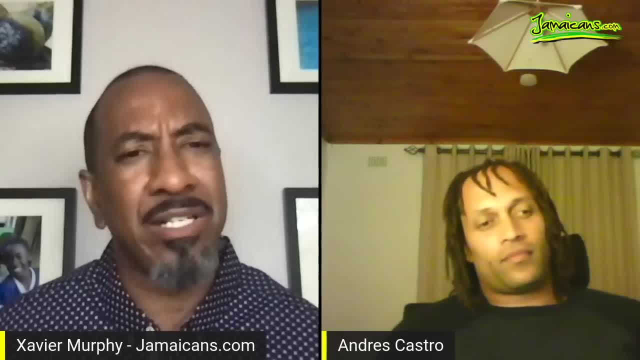 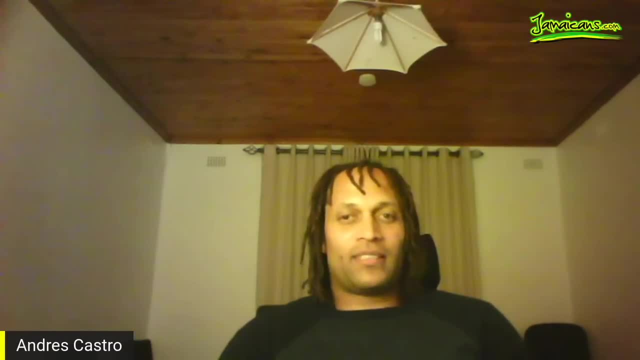 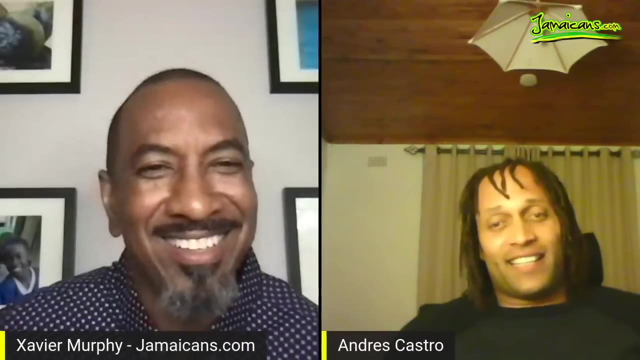 a school. you go to an and and learn it, or are you kind of learning it from the people around you? i'm learning it more from the people around me. so, you know, you say like makadi, you know iribo, and then slang, you go bobo. that is like a yard man's way of saying, well, go on, yeah, bobo. 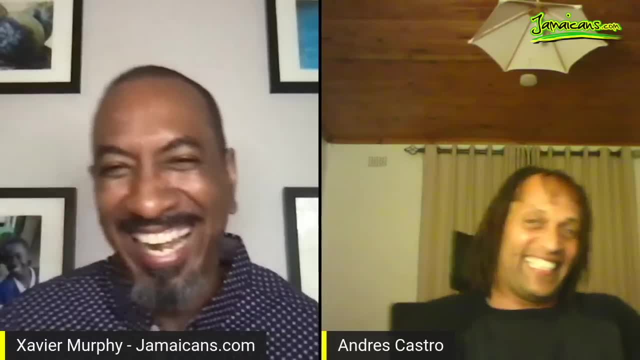 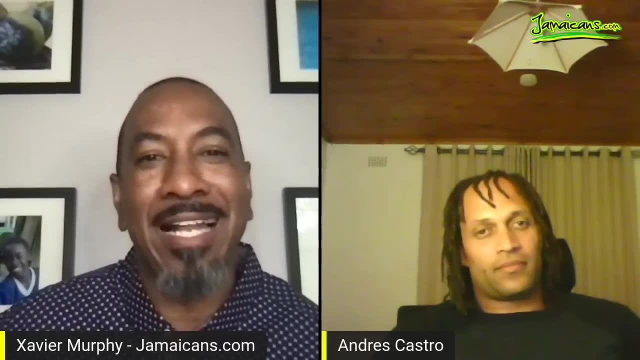 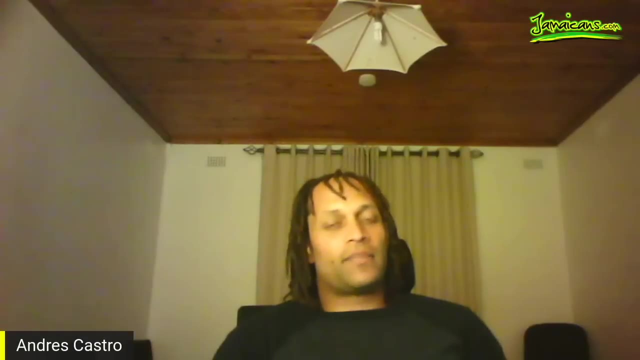 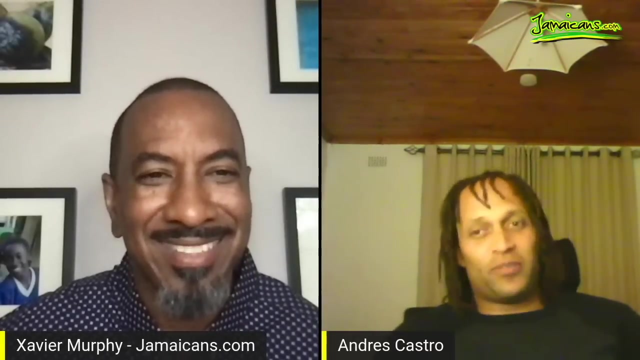 well, go on, bobo. well, we're going. we're going to touch back on the language um a little later on um cost of living. what's the cost of living right there? it's expensive. it's expensive um being Jamaican, reverse, right. so go to bar is like going to downtown for shopping or carnation market. so 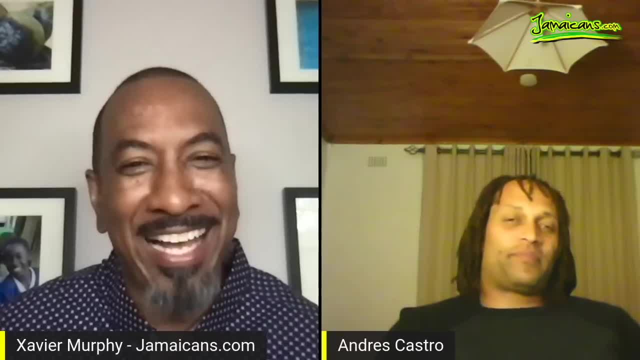 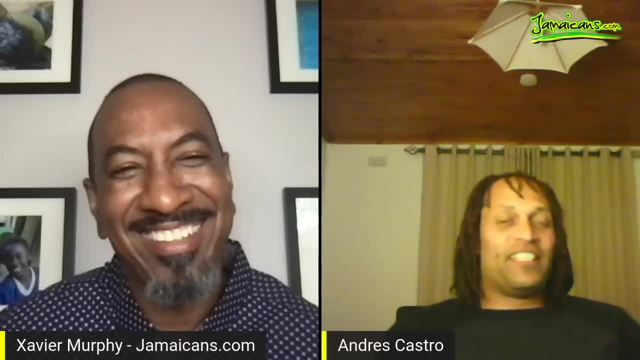 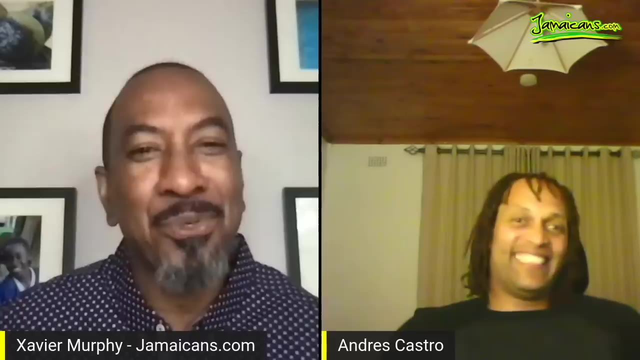 you, you, you may do with what you can find, exactly you know any yam. no, you have to, you have to go and you have to run off the plug with a Nigerian for that one. you know what about your fruits? what type of fruits you get? um, everything from grapes to mangoes. 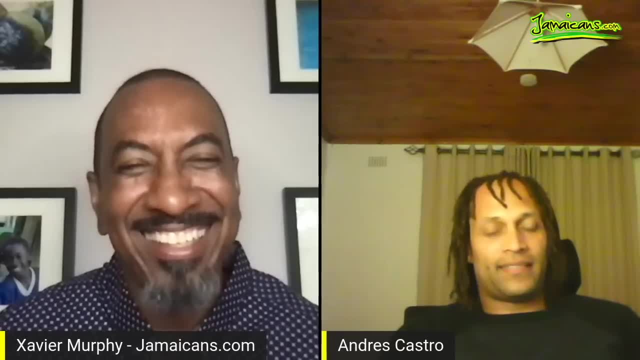 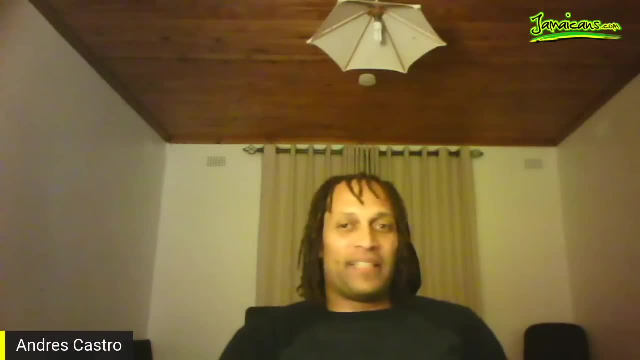 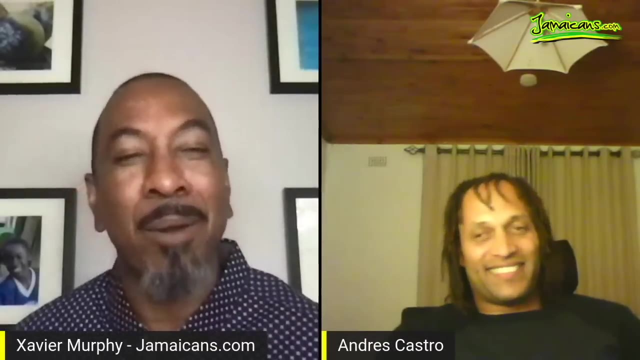 even sugar cane, all right, yeah. so as a vegan, you're a happy camper. then if you're getting at least your mangoes, you're a happy camper, I'm happy. I'm even starting to grow my own watermelon and stuff in the back garden. you know, nice, nice, but back to cost of. living. what would you say on the average meal in? you can either break it in US dollars or Jamaican dollars, if you can. what would that average meal at a medium restaurant cost? I would say between five to ten dollars. I would say between five to ten dollars. I would say between five to ten. 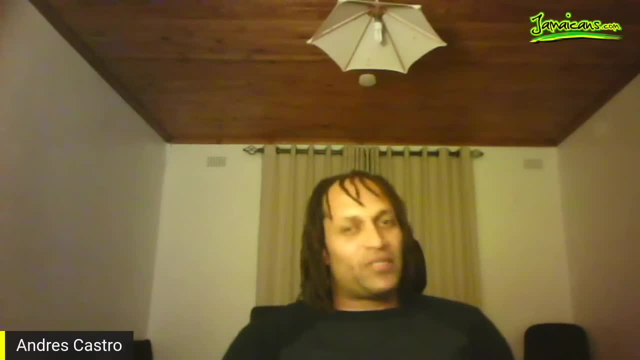 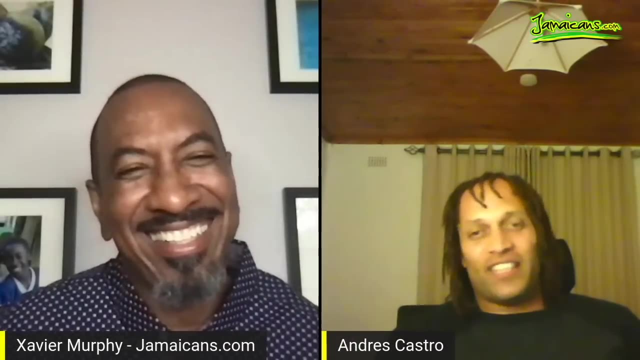 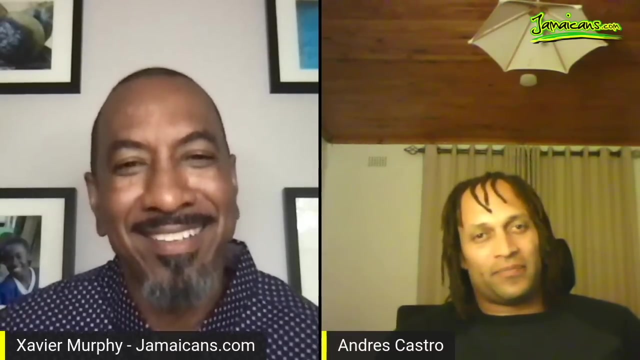 US, so not not too extravagant. it depends what what level of class you want to go to. you know, I mean, if it's, if it's if it's like the street vendors that used to buy from, then you're talking probably about two to five US. okay, all right, so I'm gonna jump in, because I said dinner. 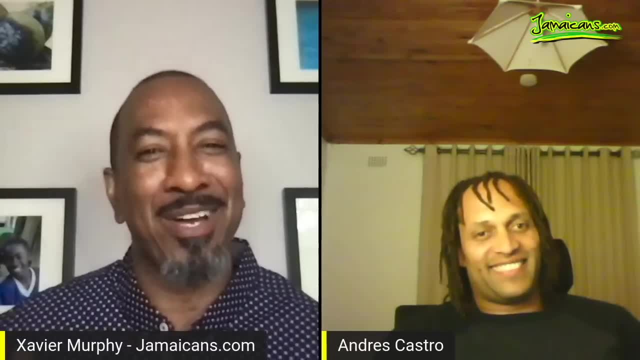 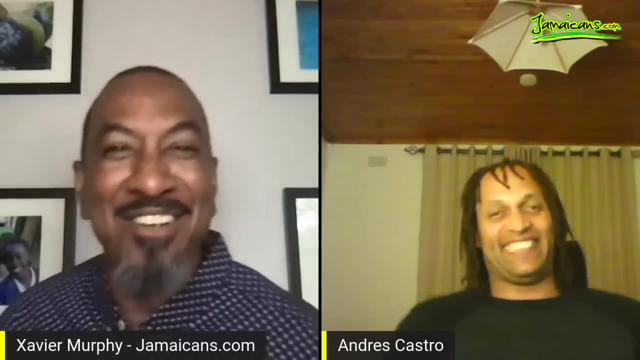 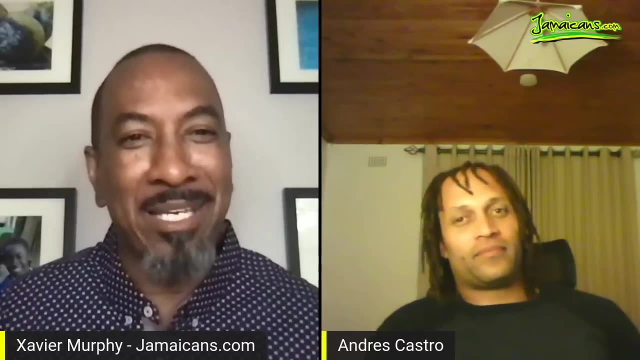 let's say, you know you're taking a lady to dinner is where I was going. but what? yeah, okay, yes, I know, sit up. you have to sit up for this one. so, um, what's the dating scene? like, I mean, you know, there is it, you know. 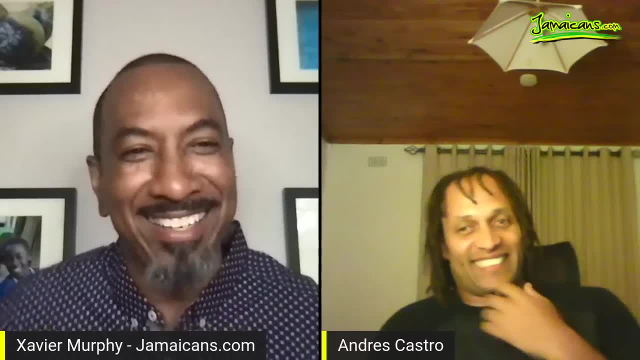 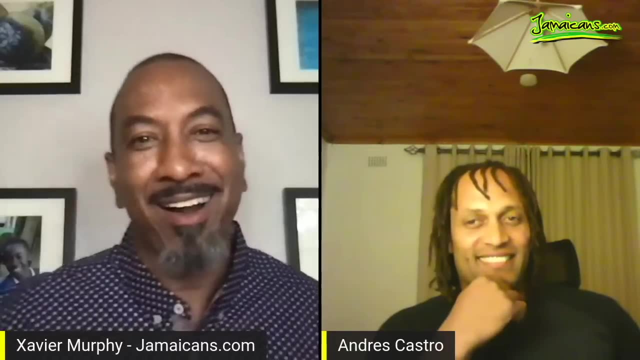 are the men? are the men, then? the men checking a lady? are they blatantly aggressive, like they said Jamaican men are? are they more subtle? and what are the women like? and again, I don't want to get you in trouble, you don't have to answer. you can please answer me if you want to. 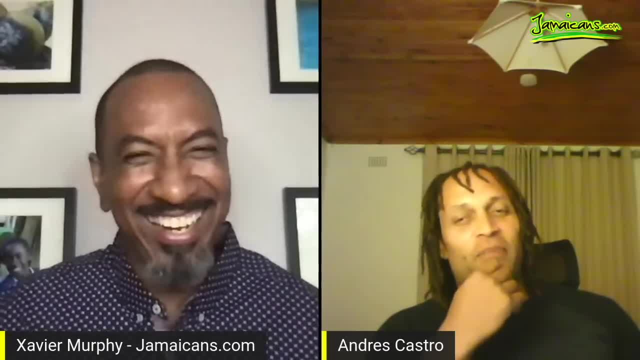 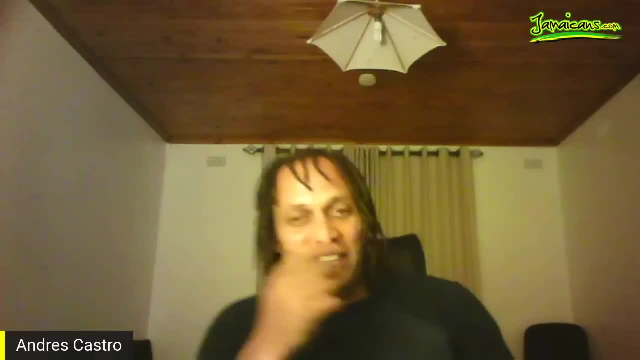 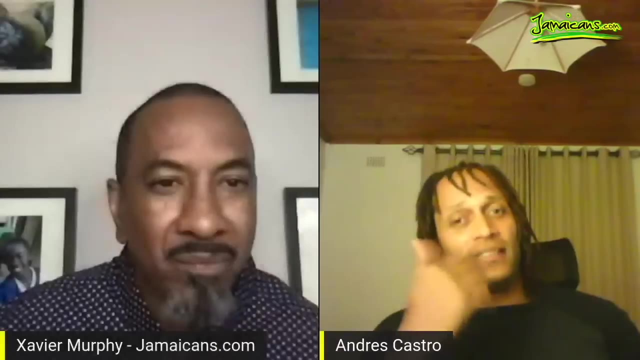 well, I'm not pleading the fifth from from what I've heard from friends. what I've heard from friends is: they're very subtle, um, and I think, if they like you, the women will approach you and guys vice versa for women, oh so women will come up to you and say: 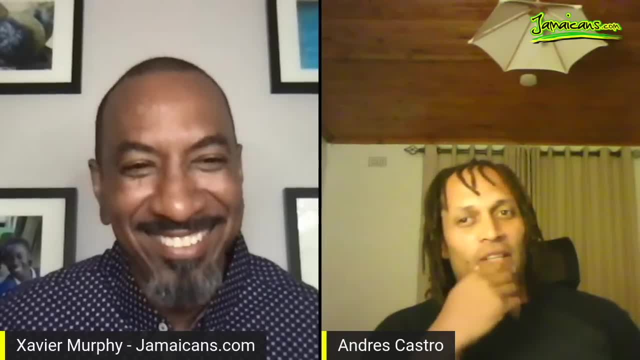 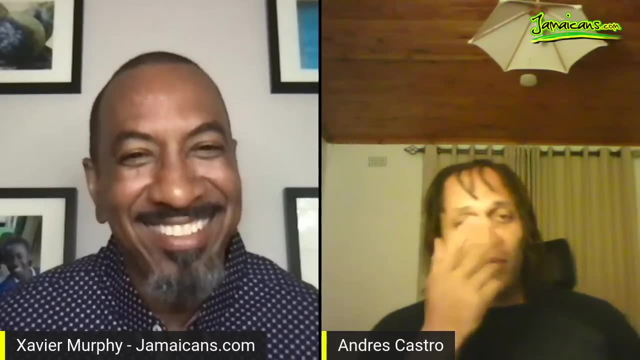 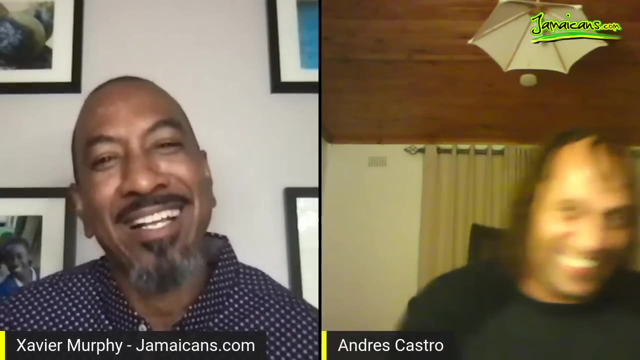 I like you. well, not that forward. where are you from? you know I? I normally get it because you know they look at me and as a brown man, so they'll be like you. sure you're Jamaican, I'm like, you know. and then then, when you tell him your name, Andres Castro. 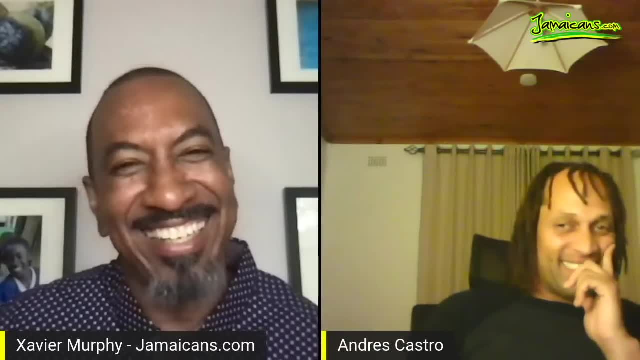 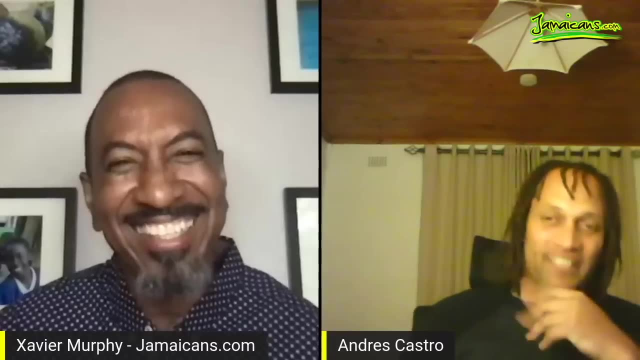 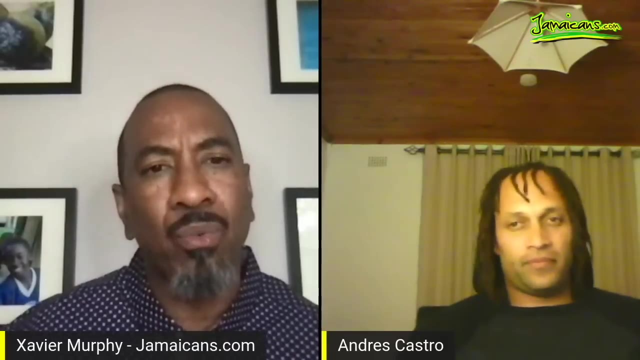 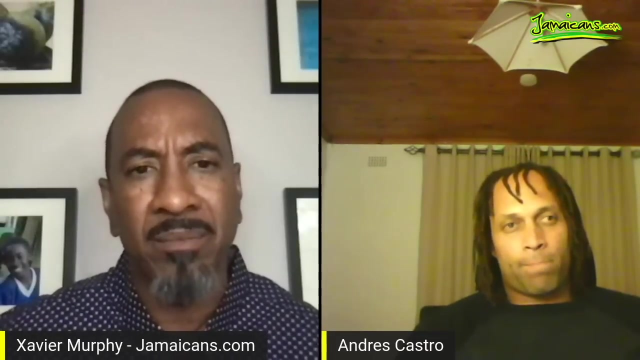 it's a different plug, you know, you know they're like, you're sure not from Cuba or somewhere else, that's it. you know the Spanish bloodline is there, but you know, right, right, all right. so what would you say for you? what was? was the the the biggest adjustment you had to make? moving to Zimbabwe? um? 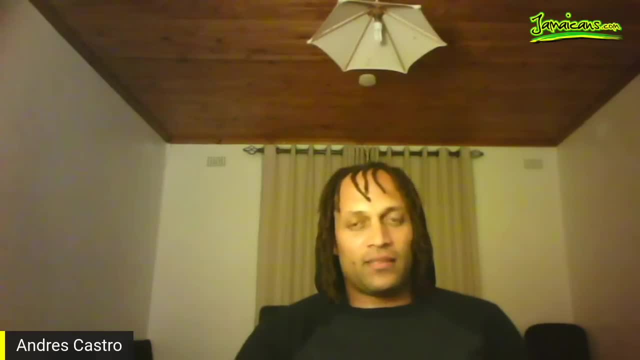 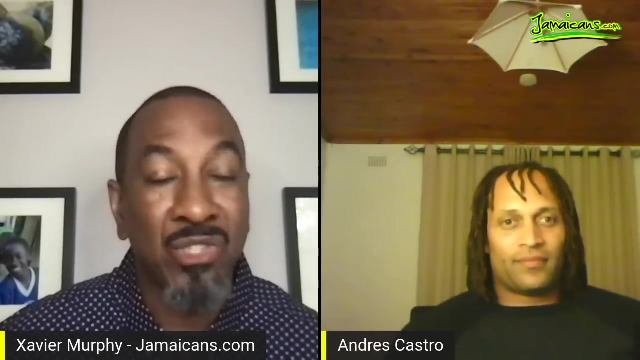 for me, I, I think it's adaptability. you, you, you go in with an open mind, um, knowing things are rough, but you learn to adapt and I think, coming from Jamaica, we adapt quite easily to to too many things. uh, anyway, yeah, I, I can attest to that, after doing well, so many of these interviews, how we, as Jamaicans, just 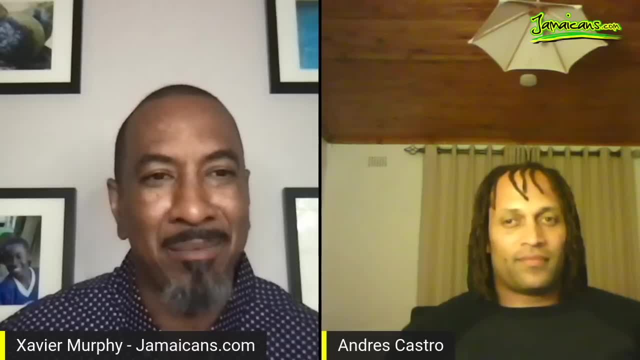 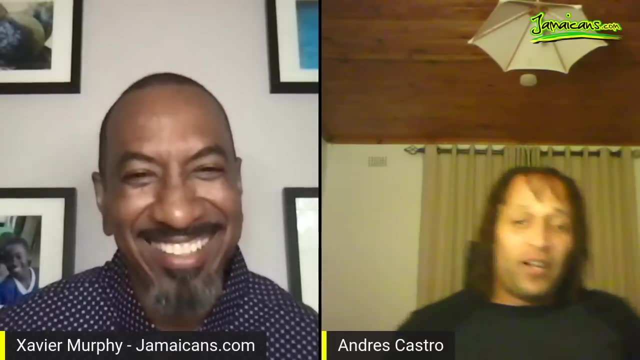 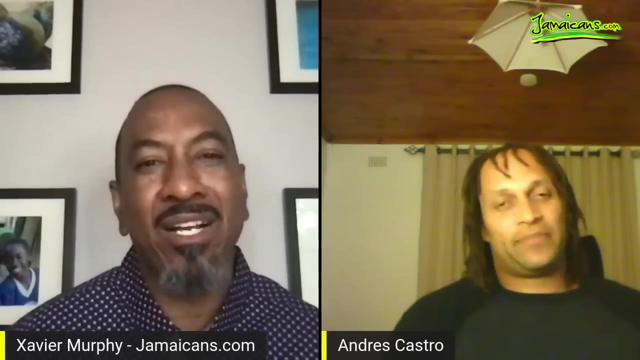 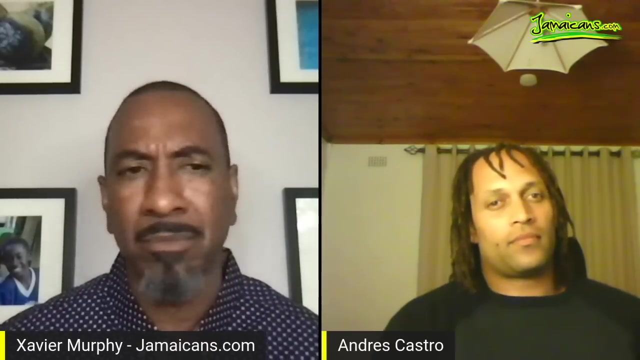 you know, we got to a place and we adapt and and um excel and, as I always say, we jaminate or we move it and we say we're up topping it. you know are are there any customs that you found when you got there that you said: this is very interesting. it can be. you know anything i've heard people say: 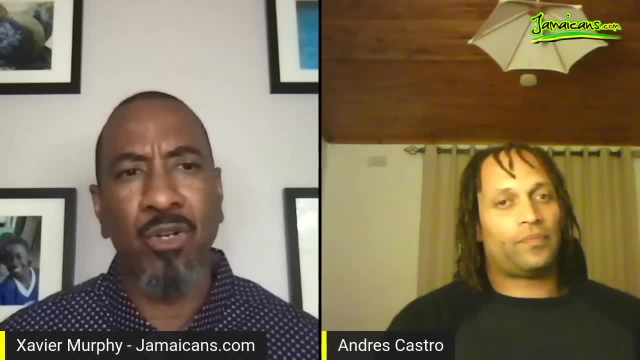 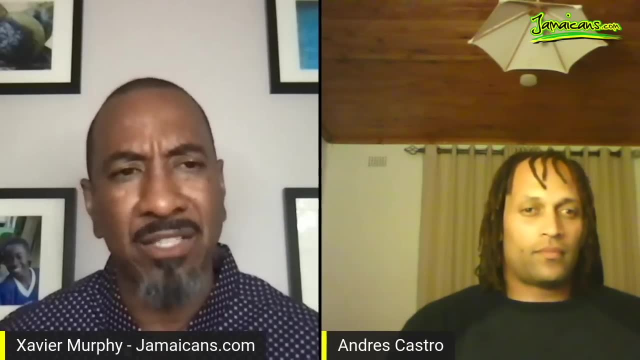 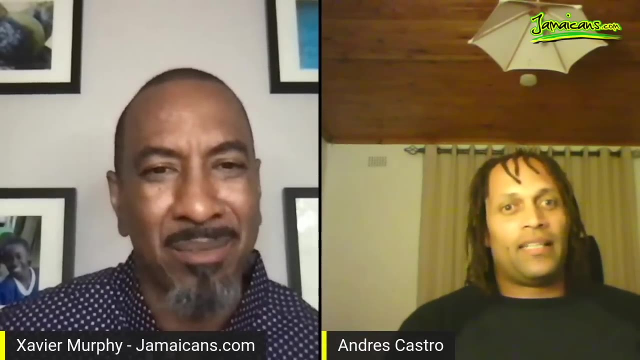 the way weddings are done, the way you know you may introduce yourself to someone, or maybe during christmas their christmas custom is different, or they are celebrated, you know. uh, so anything you can think about that you found very interesting in terms of it's, it's- i think it's, it's quite. 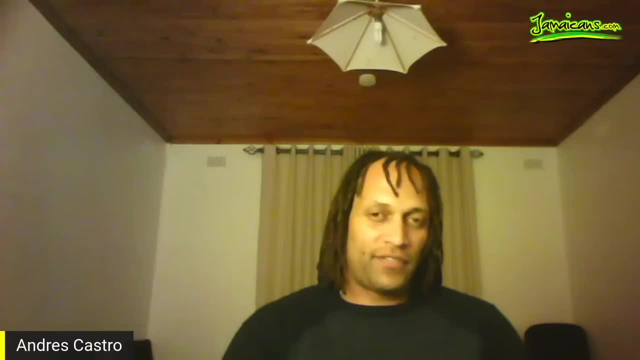 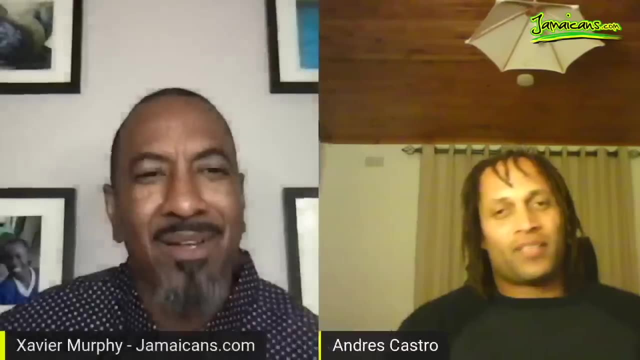 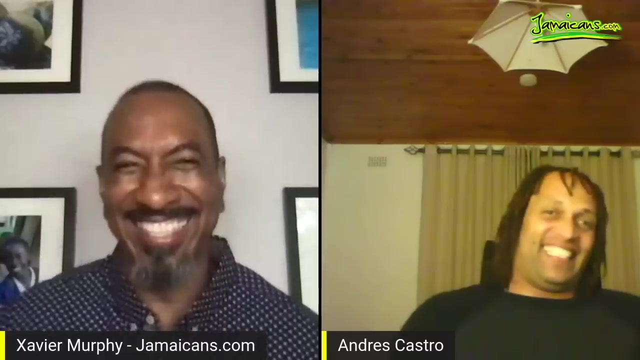 similar to jamaica the level of respect you give the, the grandmas, which they don't say grandma. here they call them gogos, but um gogo, gogo. but you know, gogo means something else in jamaica, that's why i'm looking like gogo. 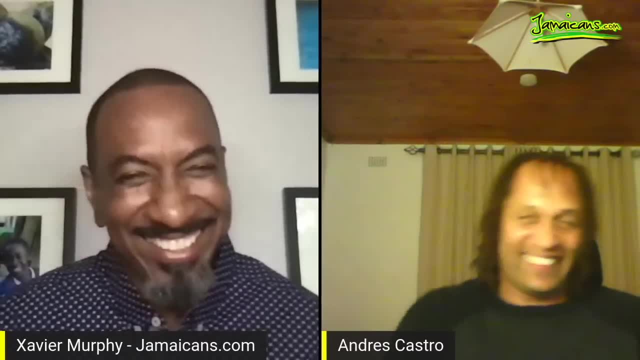 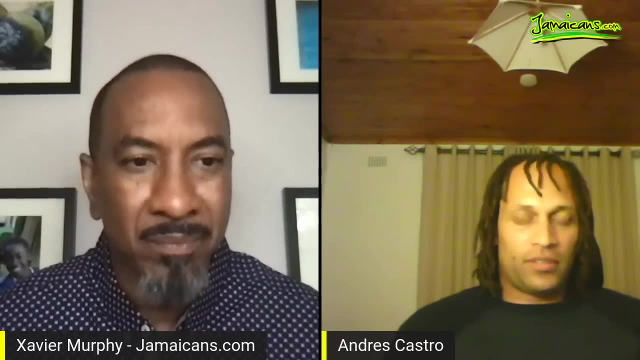 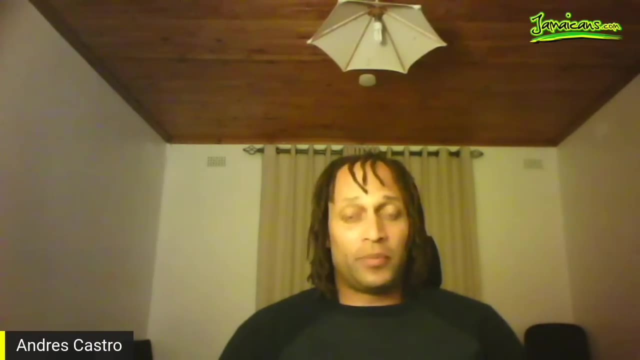 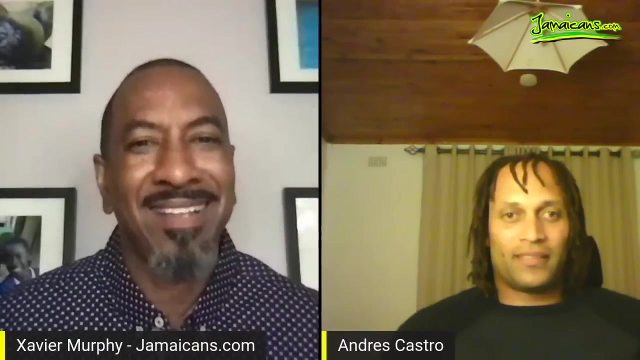 so you're saying the level of respect for grandmas, and when you go into a house, you all the males have to sit on one side and the female sits on one side. if you're meeting new, new people or new family, that's tradition. um, so i i learned that pretty quickly, okay, yes, so when 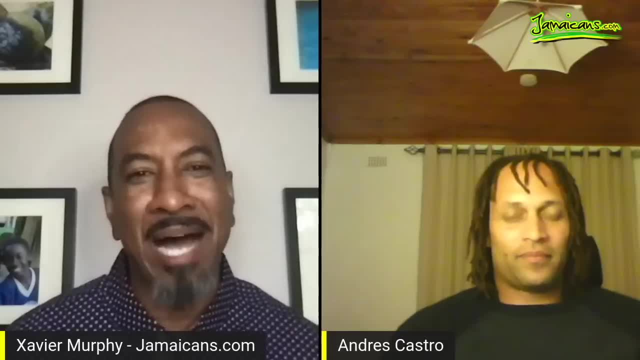 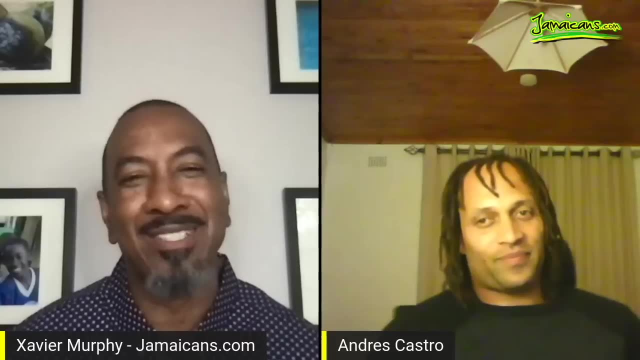 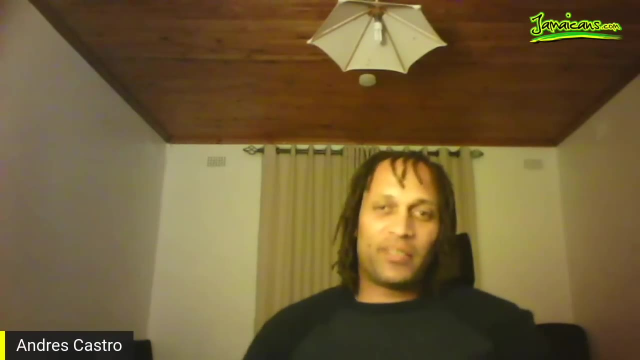 you're a busy man. when you're not busy, what is that thing in zimbabwe that you say? you know i have two days, i have a couple days. this is what i'm going to. you know, i love doing here in zimbabwe. so for me i i tend to try and go on the spiritual realm and try and go and walk in the mountains, um. 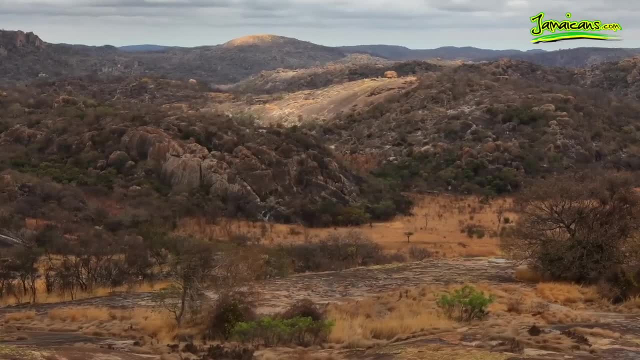 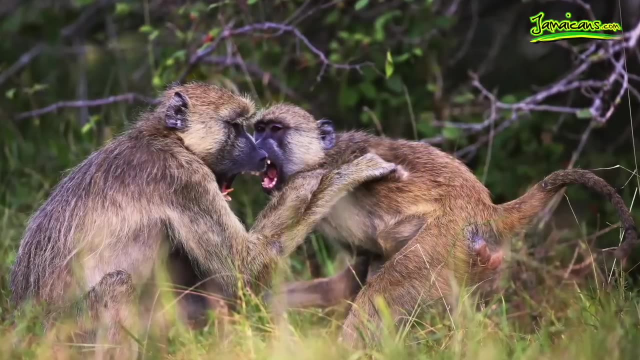 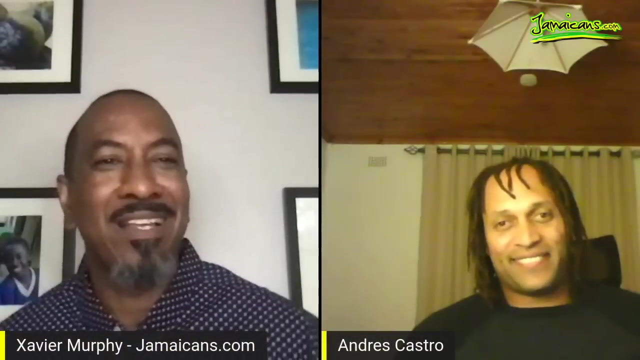 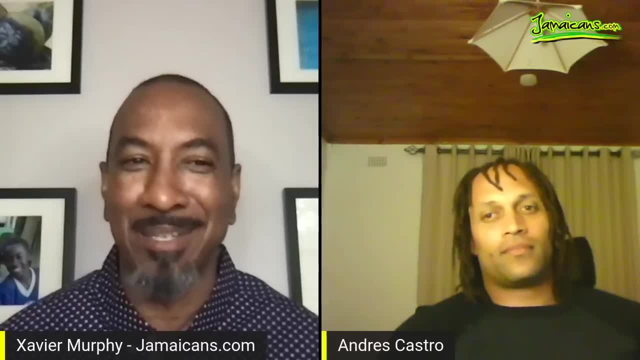 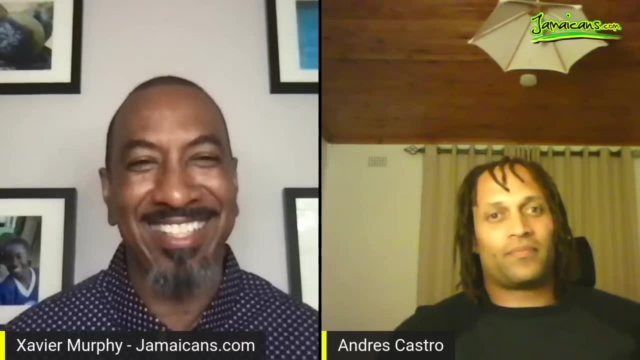 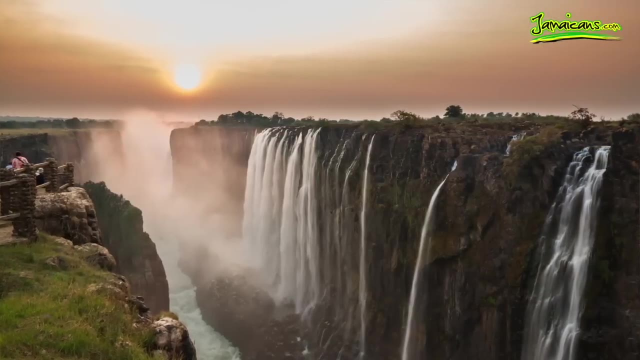 I don't want to jump ahead because I think I know what you're going to say, because Zimbabwe is known for it. but the one place that folks should visit in Zimbabwe, what would it be? Well, everyone says Victoria Falls, but there's Nanga, which is in the mountains. 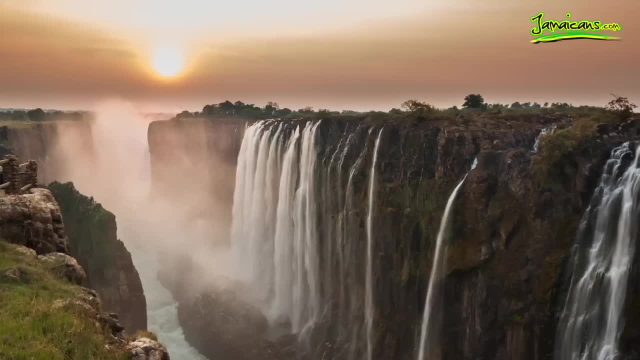 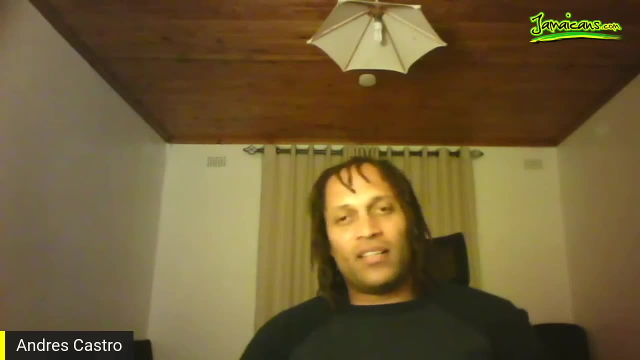 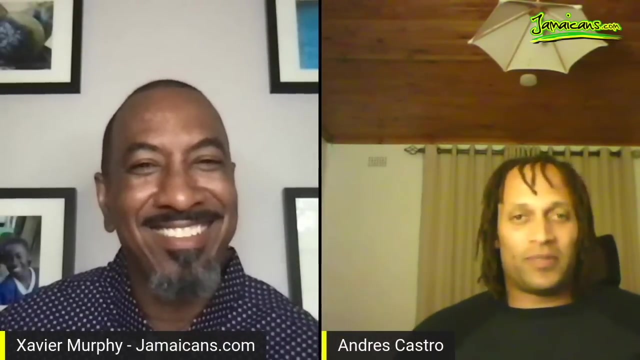 Nanga is in the mountains- what's the best way to describe it? It's almost like Blue Mountains, but you have rivers and lakes and there's a waterfall there. so I would say for people to go there, they have Kariba. but when I went to Kariba, 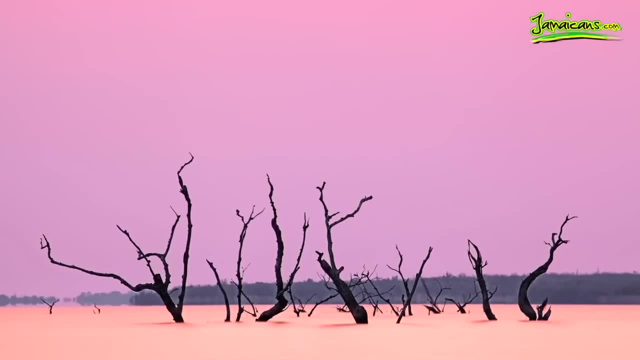 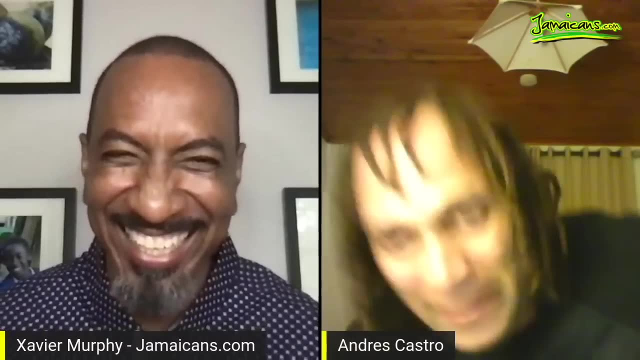 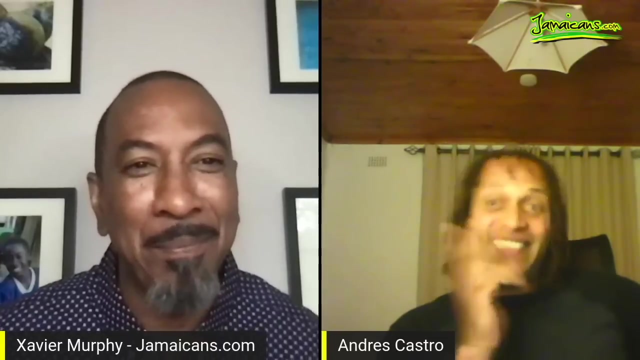 a friend was like can I go and swim in the river? and he's like: no, there's crocodiles in the river. I said good thing you asked a question, because some people see water and they just jump, jump in the water. you know, coming from Jamaica, 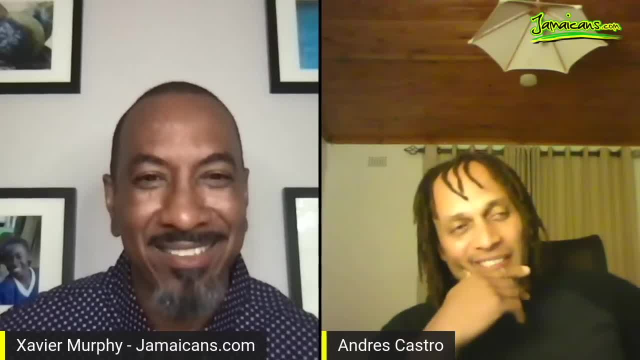 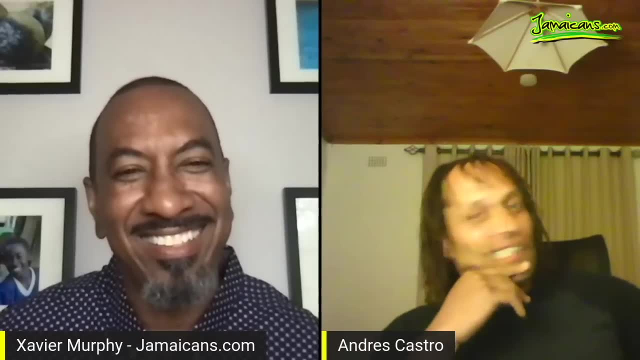 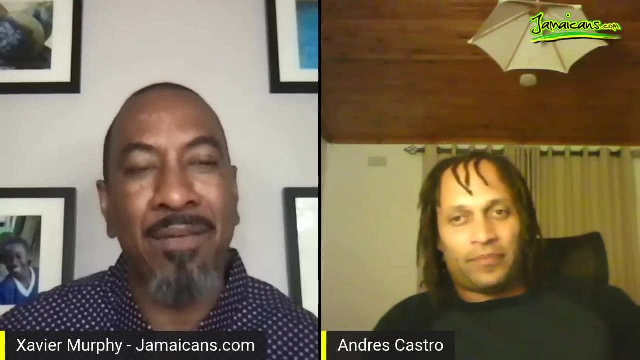 we used to see crystal clear water, right. so you go in there and you can't really see underneath the water. then you start to see hippos in the water. you start to double check yourself so you're in nature. it sounds like if someone loves nature, it's a great place. 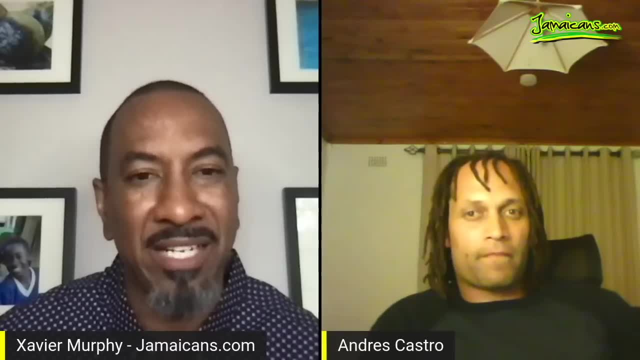 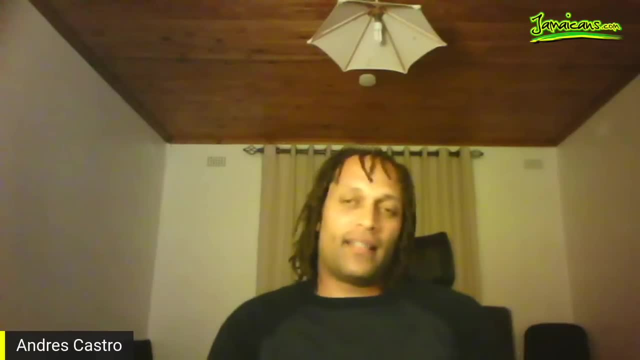 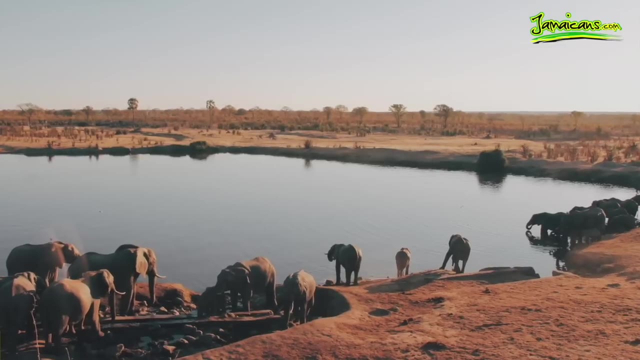 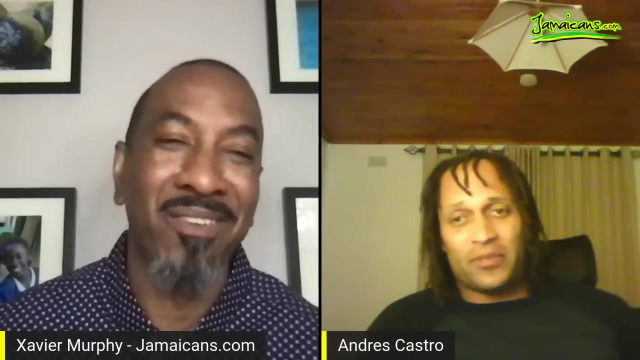 to hike and a great place to visit for nature walks and so on. definitely, there's what they call loads of game parks, like reserves, where you can go and see loads of animals like elephants, lions, hippos and and wild boars, you know. so how do you get? 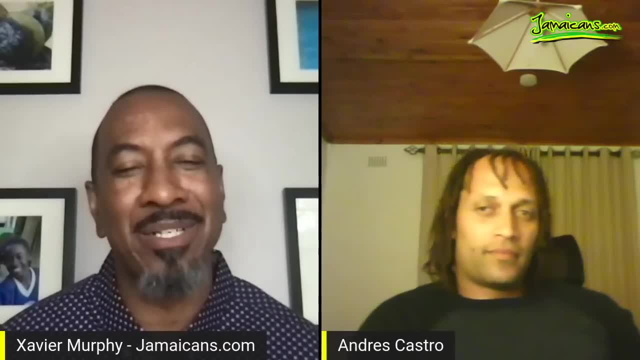 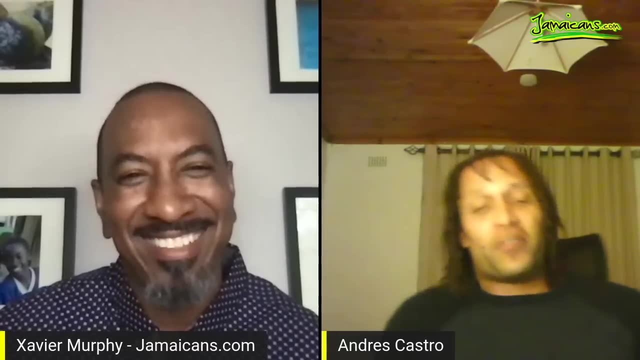 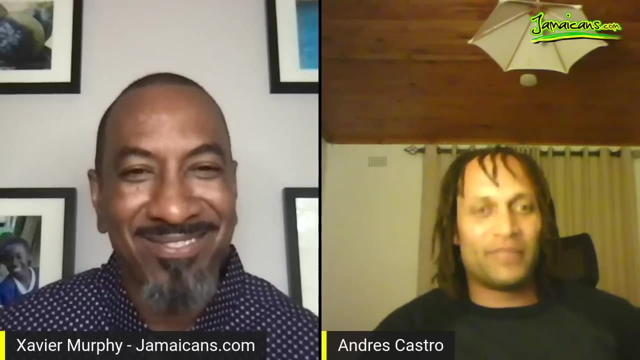 I know you're vegan. how do you get your Jamaican fix now? is there any Caribbean Jamaican type restaurants there or no? no, no, I cook for myself and I cook for friends, you know. so I always make sure my seasoning is with me, you know. 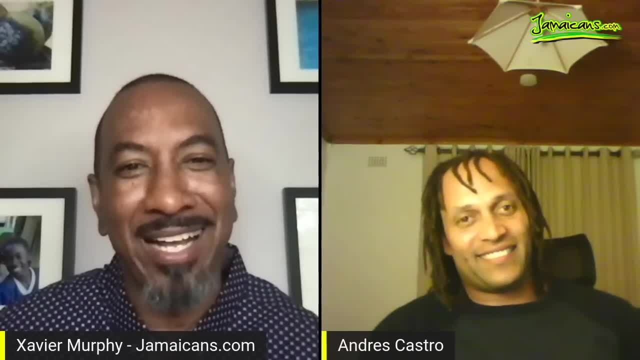 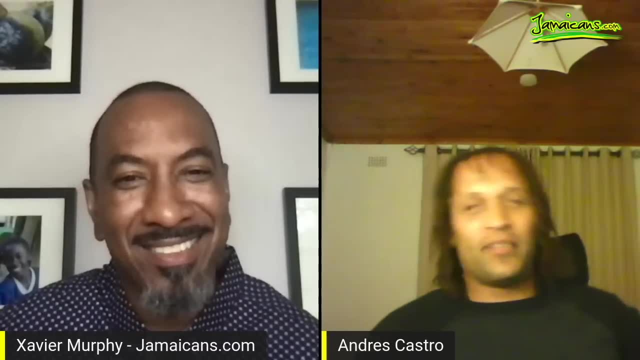 and what do they think when you cook the Jamaican food? I don't know if you get any ackee or any of that there. no, no, no. so when I travel again, you know, because I'm due back a visit back home soon- so when I'm travelling, 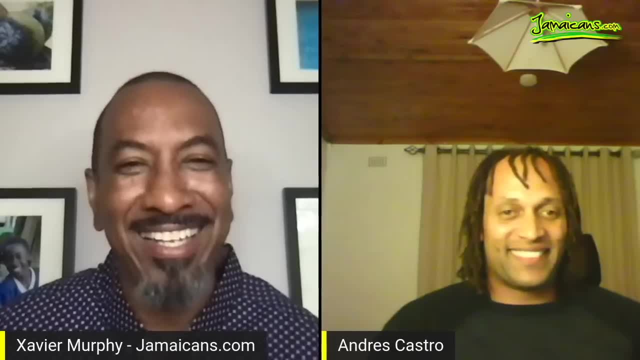 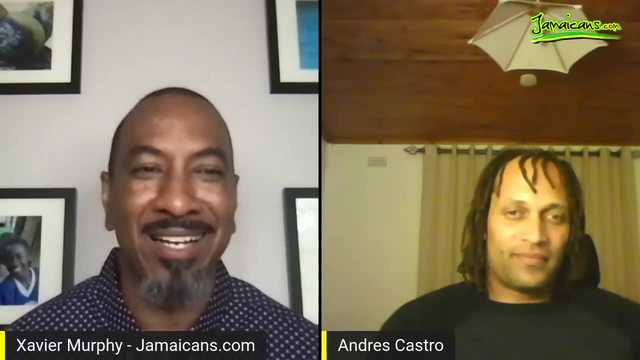 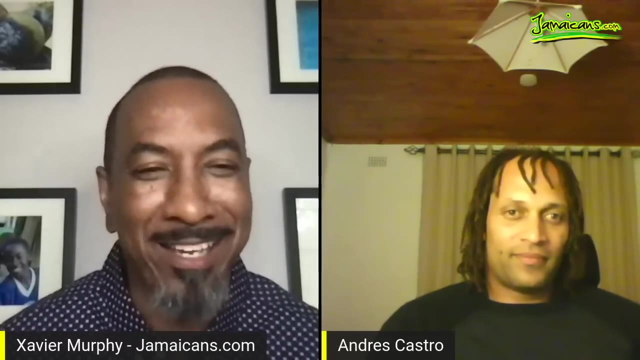 I'll stock up and I'll go to the Jamaican restaurants, you know, okay. so that leads me- and listen, Andres, thank you. thank you for providing us with, you know, insight in Zimbabwe. so it leads me to this question. a scenario: you land in Jamaica. what is that first thing you're doing? 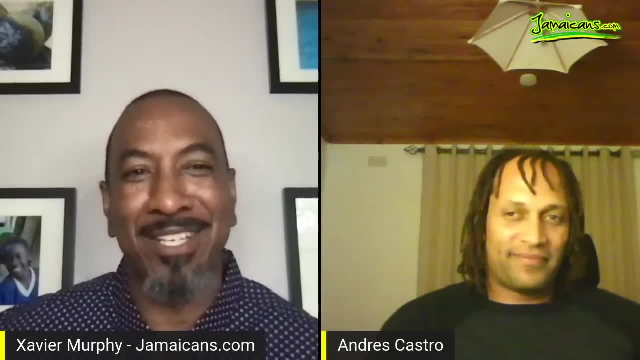 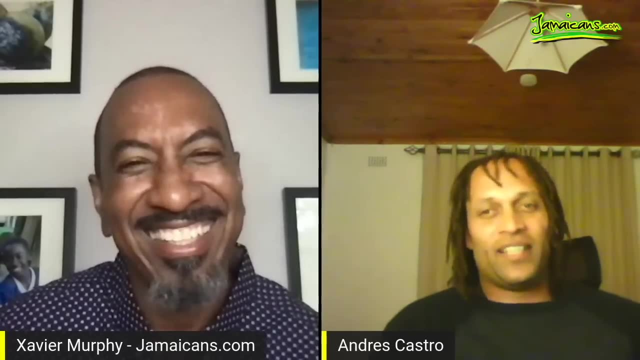 when you get off the plane, or that first thing you're going to eat, or that first. you know, everybody has a different thing when they get out, well, you know it's the first thing. well, I have to see my mummy because you know mummy is important. 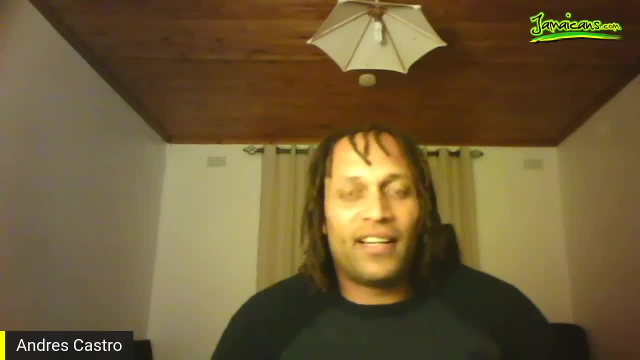 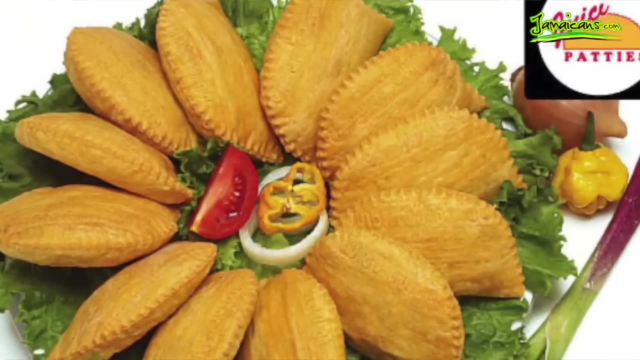 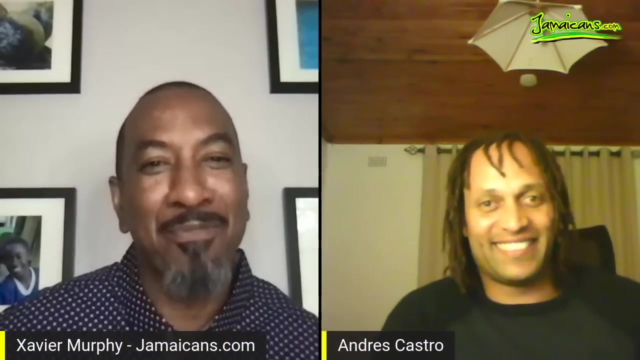 for me it's probably have a nice veggie patty from juicy beef patty, some coca bread, you know. all right. so, folks, you know, if you're visiting Andres in Zimbabwe, please take him a veggie or a cup of veggie. freeze them. take him a cup of veggie. 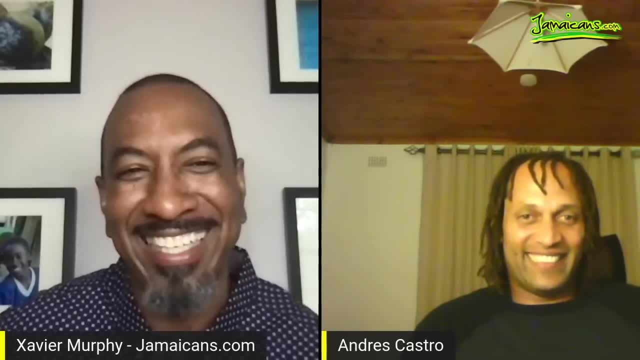 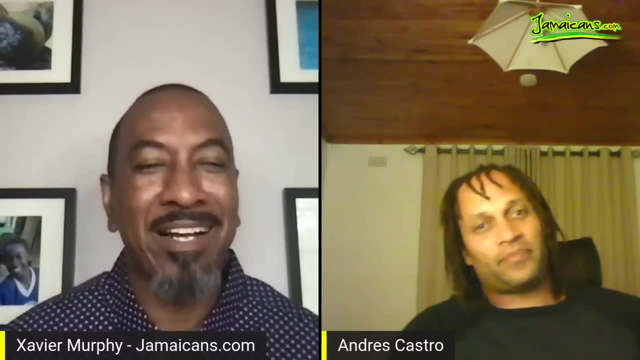 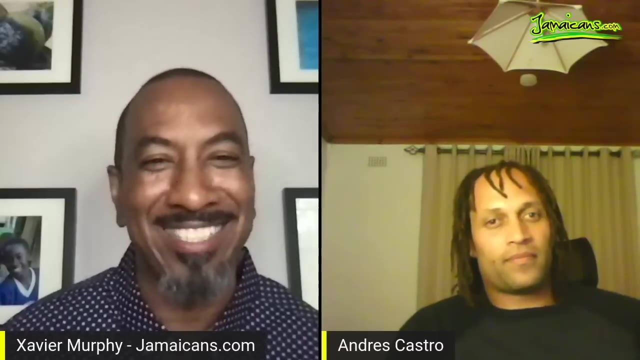 juicy beef patty with some coca bread. that's what we're going to do. so here is how I typically end, how, and I think you kind of gave me the hello, the what's up. Bobo, I think it's a what's up. so well, you normally say: 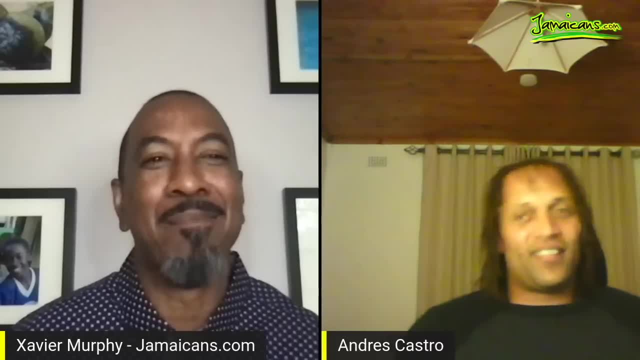 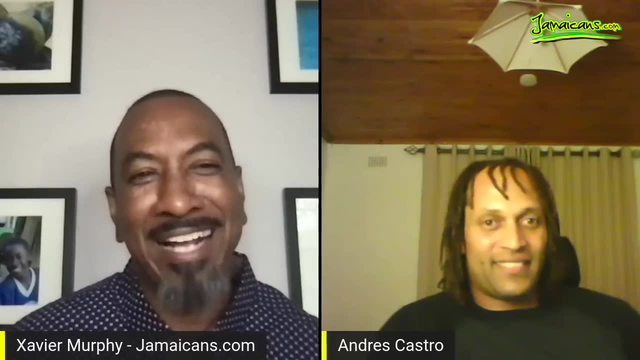 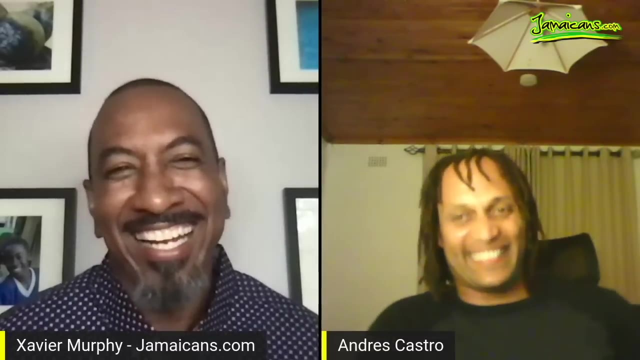 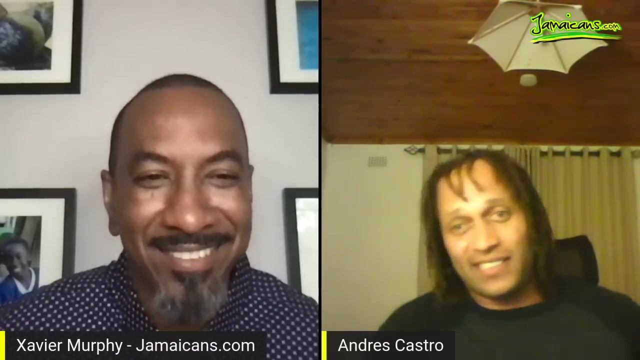 makadi, which is like hello. it's like our Jamaican way of saying wagwan, wagwan, makadi, makadi. so can I add: like makadi, my brethren and I like a patwa swing swing to it. you know, the funniest thing is in the getter areas here. 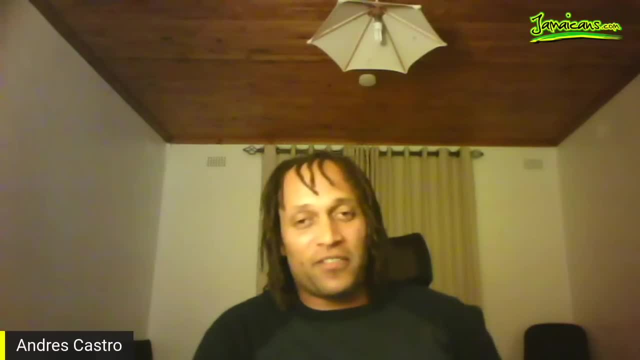 right and we have to give grateful thanks for, for Bob, for opening Jamaica to the world and I think it's transcended since then that Jamaican music has carried on in the getter areas. dancehall is very important. we have friends, we've got the You is beat and the regular. 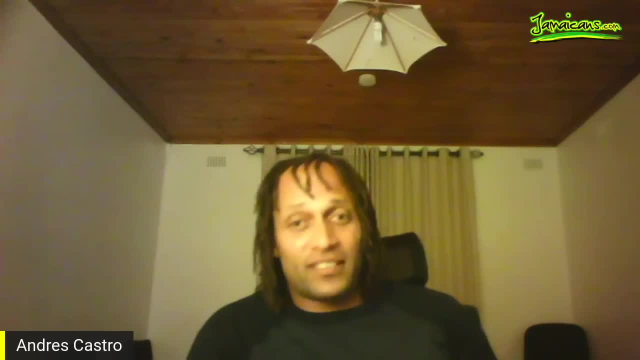 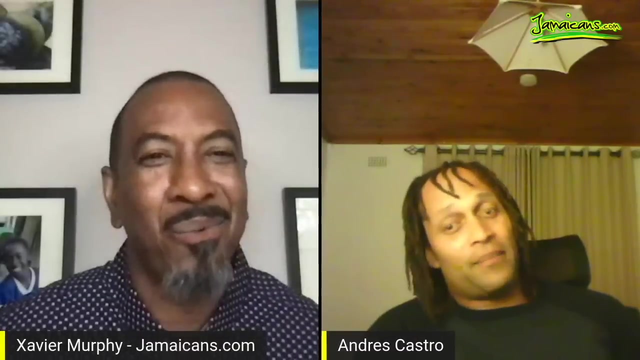 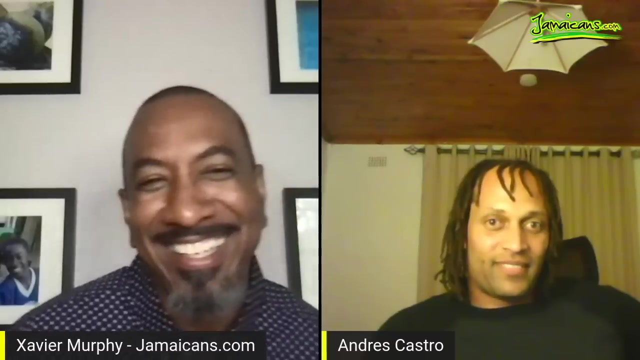 you know our friends- and I'll have to shout him out- my friend who is Nutty O, he's one of the biggest dancehall artists here in Zimbabwe. man testify, I tell you what me and them can come to Denver was important big time. you know them upset them off, them have are wait, wait and yellow intense in advance. 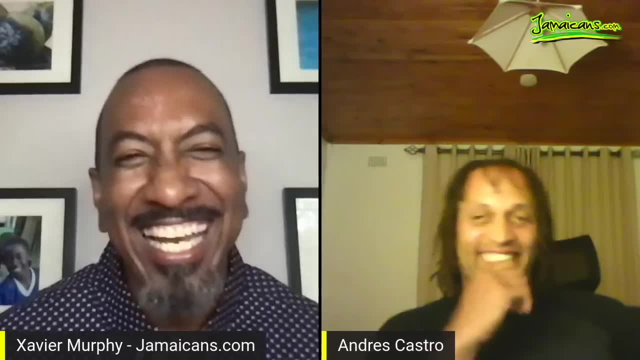 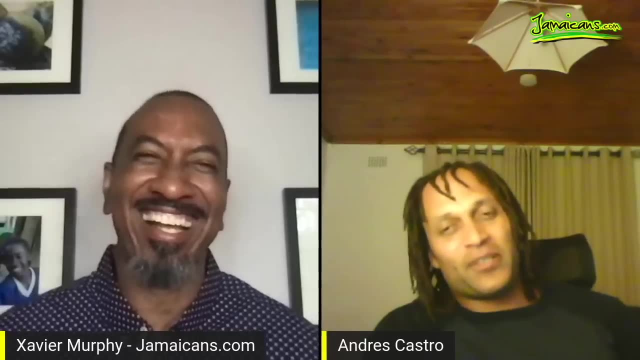 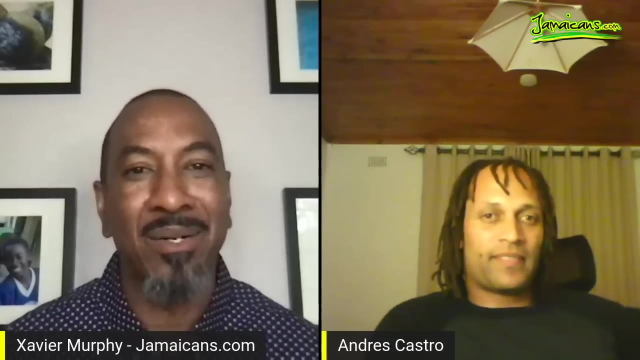 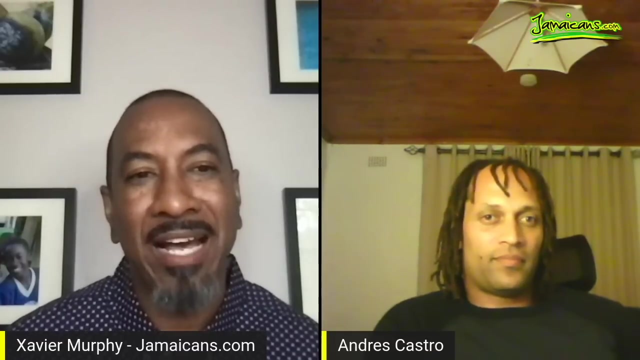 for it coming though. it coming, it coming, it would be a good, it would be a good look. you know, yeah, amazing how the music has and transcend, transcended. you know, um, i always, often, said my friend from zimbabwe says to me that we don't know what we have, we don't know. 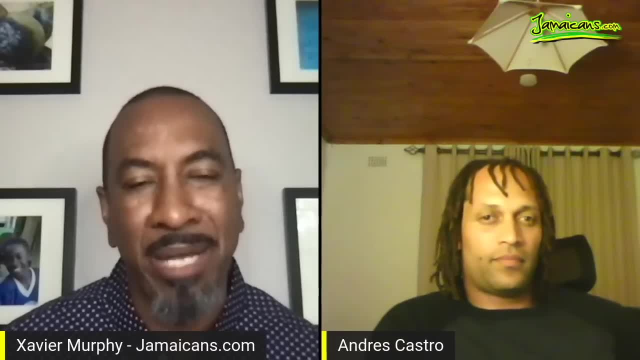 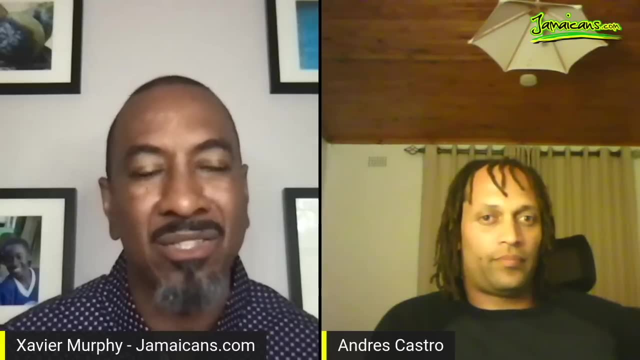 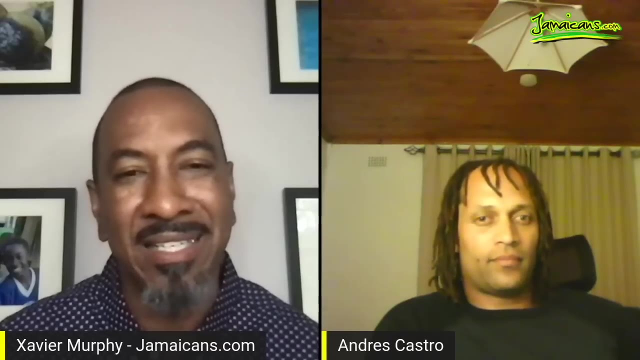 how the music uplifted them before they were independent. you know he said sundays, sundays music was. was bob marley, peter tush, burning spear, that was what they listened to on a sunday evening. and he says that music freed our mind. and so um zimbabwe, yes, 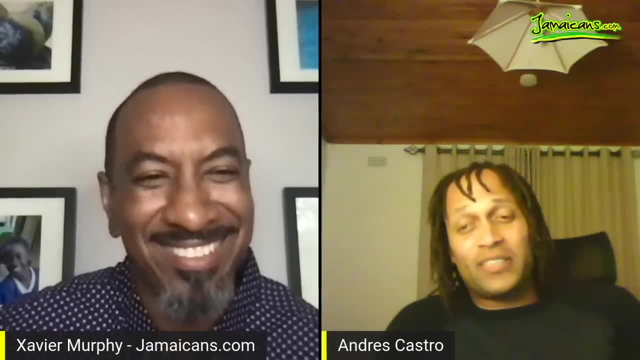 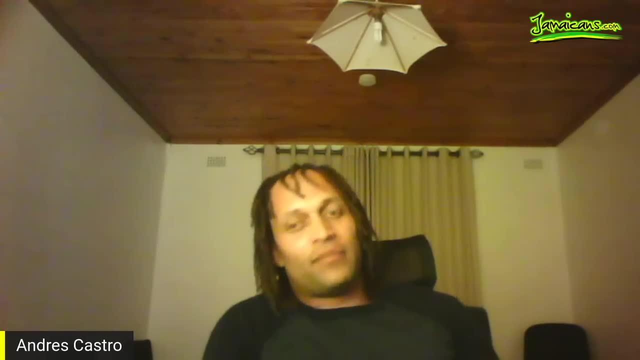 well, even even now. you know there's the busy signal, there's the kabaka pyramid- um, you know i'm gonna be biased, dennis brown is mine- but also you know the islas and the capeltons. that is vehemently beaten out in the ghetto streets in barry. 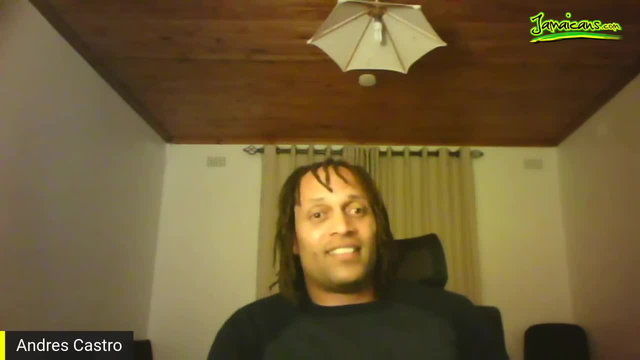 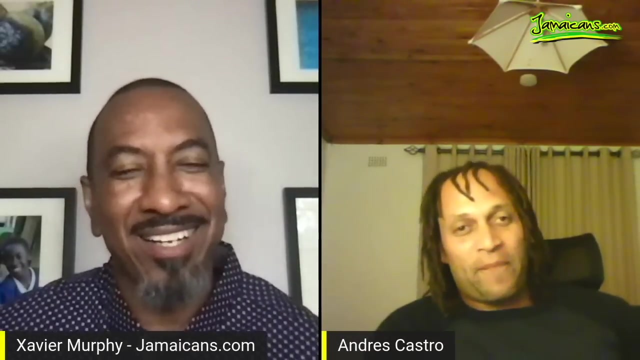 you drive down, you're leaving here some maseca. i i just introduced a few of my friends to some idonia, you know, because i like idonia as well. so it's introducing, just keeping them up to beat with the the latest dancehall. you know, you sound like you're a kind of a connoisseur there, you're, you're. 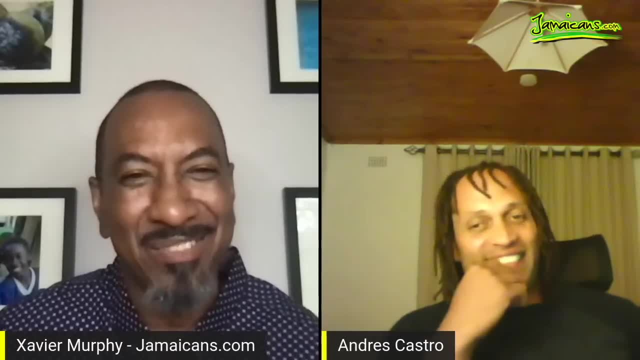 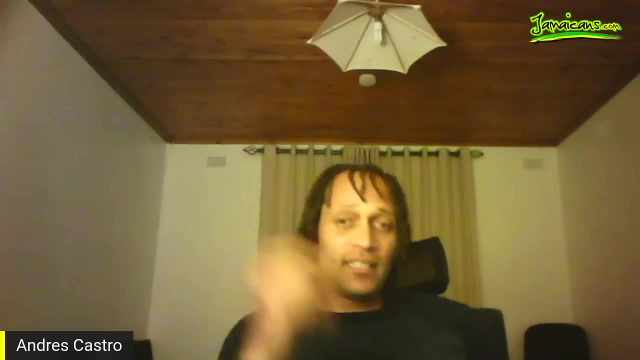 you're deep into it, my friend, definitely, definitely, you know, and and, and i think it it's, it's a big, intricate part. i was discussing it with um, some of my friends back along that do shows and you know, doing investment and i'm like you know, jamaicans really need to take a stance and really come back to africa, even. 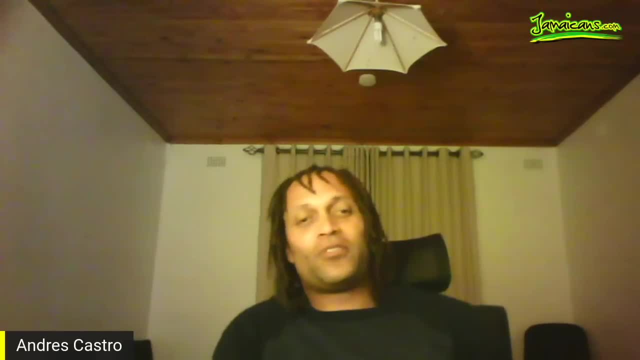 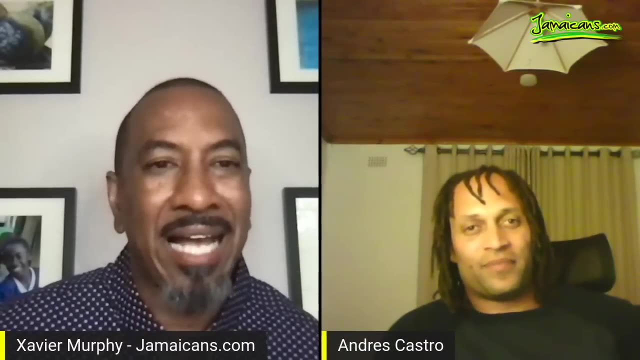 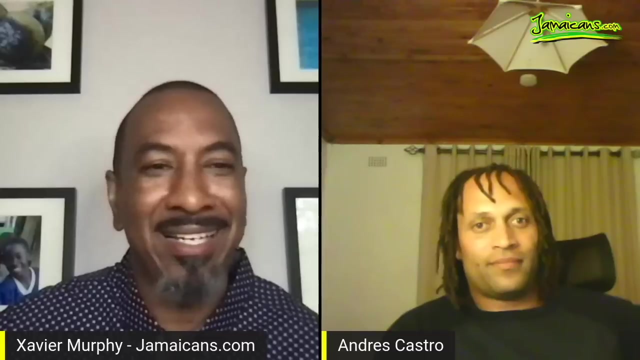 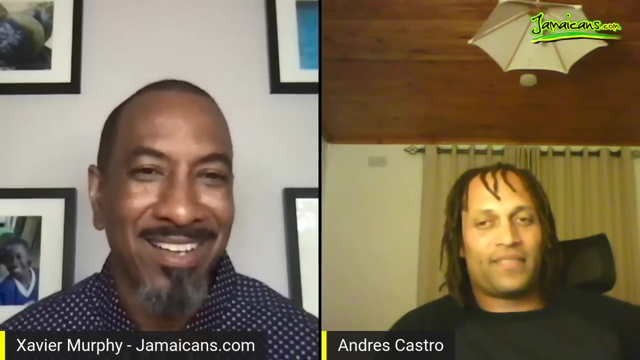 for a visit. you know, i i never knew the true meaning of returning to the motherland until you you return. yeah, i, i, i agree, i, you know i did a visit and, uh, can't explain i i get goosebumps that time when i think of the visits. you know, it's um, it's life-changing, you know. definitely so, andres, again. 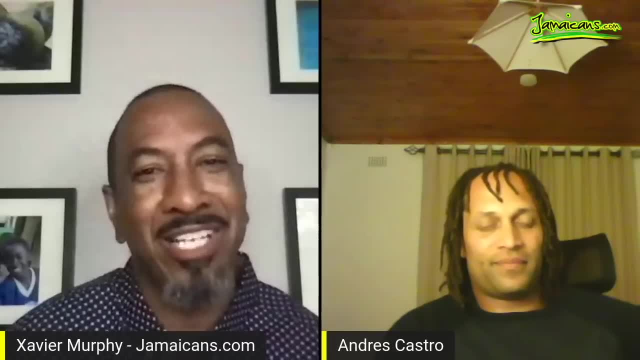 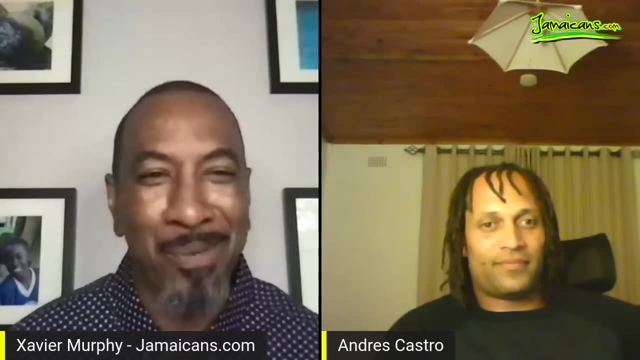 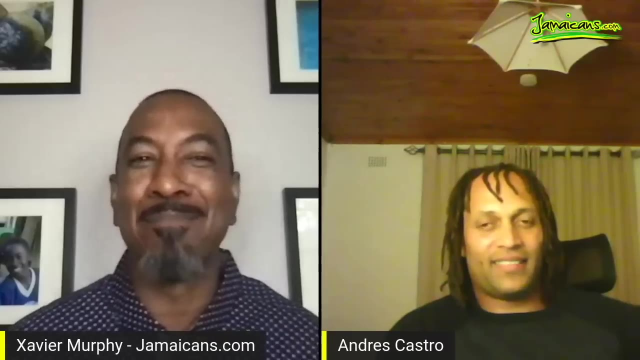 thank you. thank you for providing an insight, telling us your story. so here's how i typically end. how would i say goodbye in the most unofficial way? you kind of tell us how to say hello, um, what was it? how do you say goodbye in the most informal way in zimbabwe? well, well. 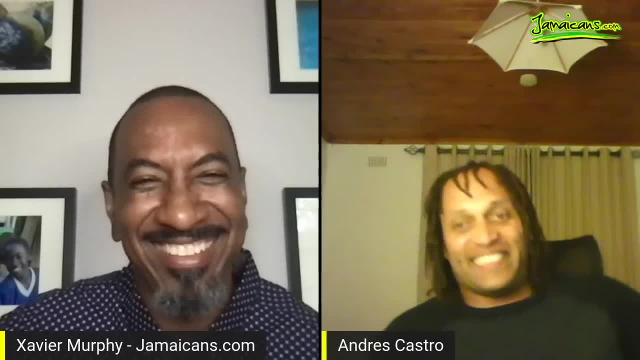 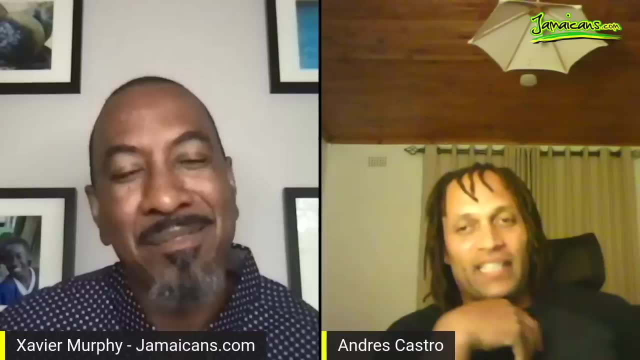 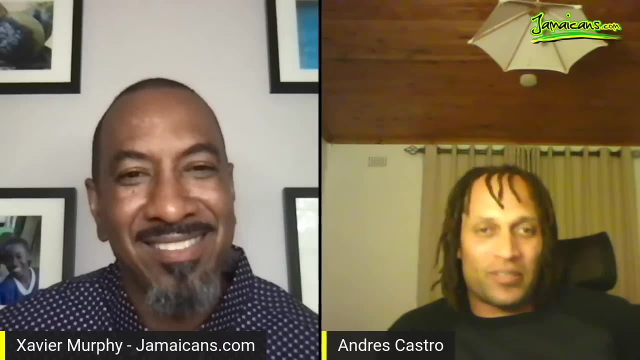 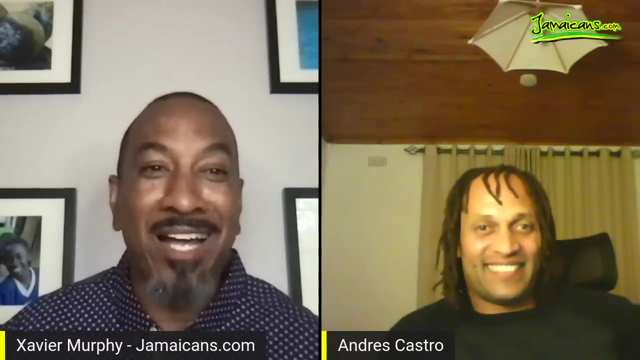 i'm gonna say nothing too bad here now you know so. so normally for me, i normally say: because i'm with friends, i normally say: two nana manguana, which is i'll see you tomorrow. okay, all right. yeah, all right. two nana manguana, my brethren, yes, blessings. 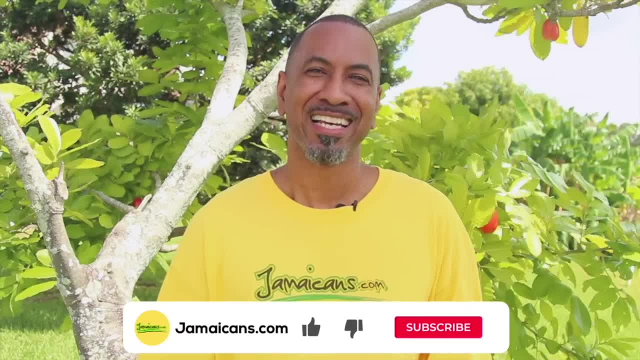 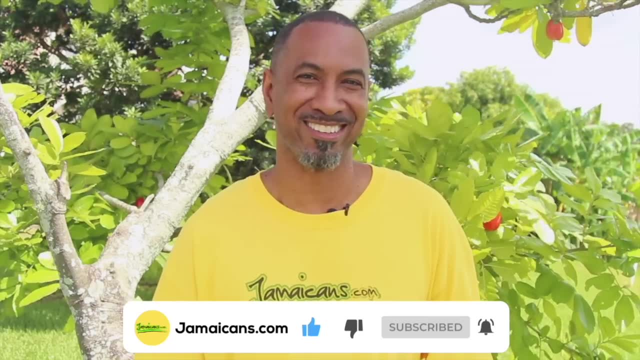 show some love now. hit that like button, subscribe to our channel and hit that notification bell. that way you don't miss a video.